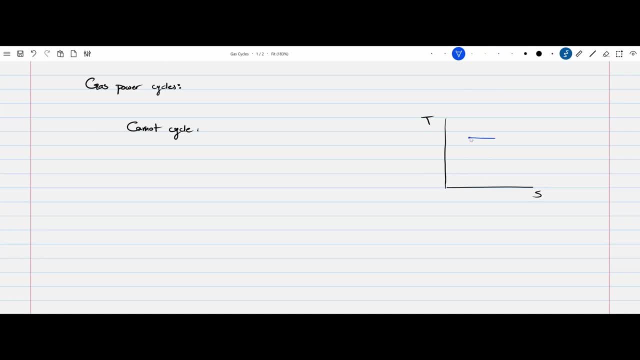 cycle. We have a heat addition process from 1 to 2, we have a work or power producing expansion from 2 to 3, a heat rejection From 3 to 4, and, of course, a power consuming compression from 4 to 1.. 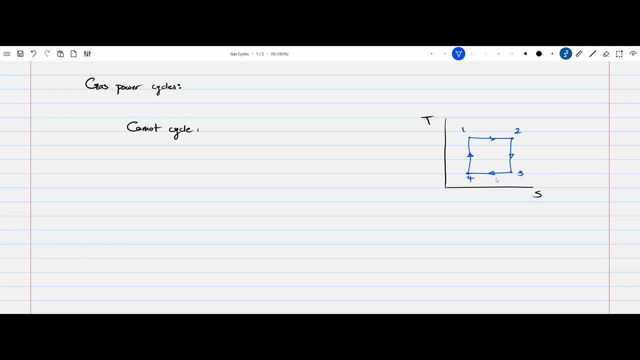 Now the thing is, this diagram represents an ideal Carnot cycle, But the issue is that the Carnot cycle, while being very useful for understanding the physics behind a power cycle, is not really practical To understand that. let's focus on this diagram. 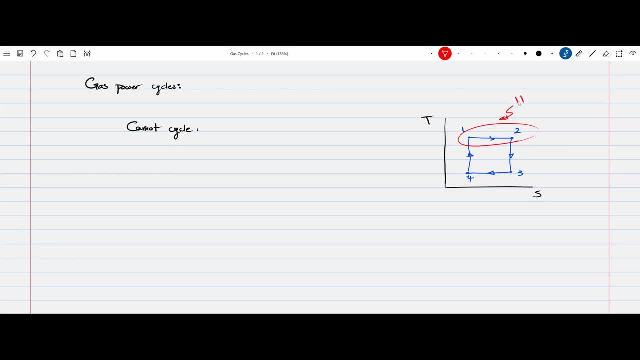 On a heat addition process. In the overview of the introduction to the Carnot cycle we will see that for the heat addition to be a completely reversible process we had to have the heat addition over an infinitesimal temperature difference between 1 and 2.. 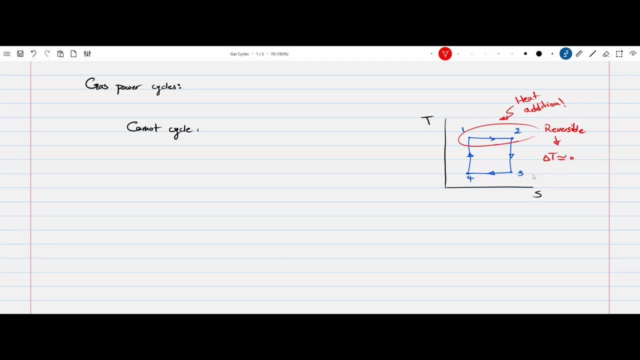 mean the system and the surroundings. That way we could ensure that the process from one to two is truly reversible. However, in practice that is not achievable. From a heat transfer perspective, the higher the temperature difference between the source and the system is, the better the heat. 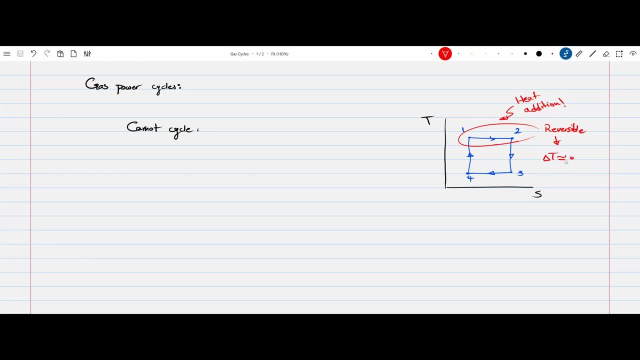 transfer rate will be. So a delta t of approximately zero is not practical. Also, if you look at the power producing expansion, you will see that in order for this power expansion to be truly reversible, we had to have the expansion at a super slow rate. 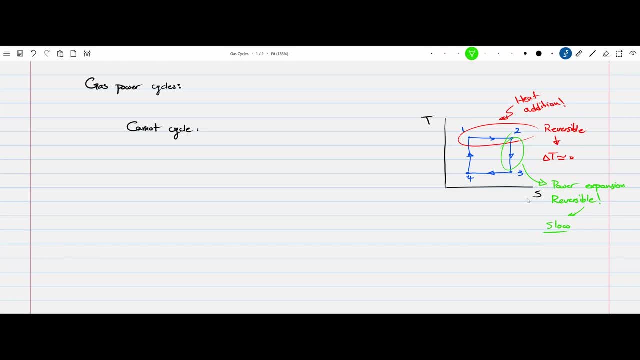 To ensure that the system and its surroundings will remain reversible. So Carnot cycle: very good for understanding the physics, not very practical in real life applications. So we have to look for and settle for the next best thing. We usually call them the ideal cycles. Now, as the name suggests, 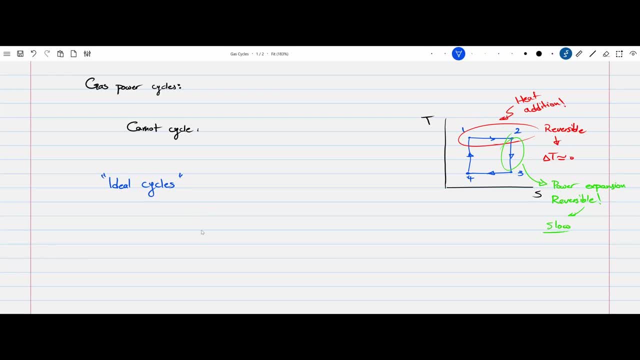 these are still ideal and theoretical. They are far away from the ideal cycles. They are far away from the ideal cycles. They are far away from what happens in practice within a system, but they are a good approximation nonetheless. We can use some of the basic understandings of the thermodynamics that we have gathered so far and 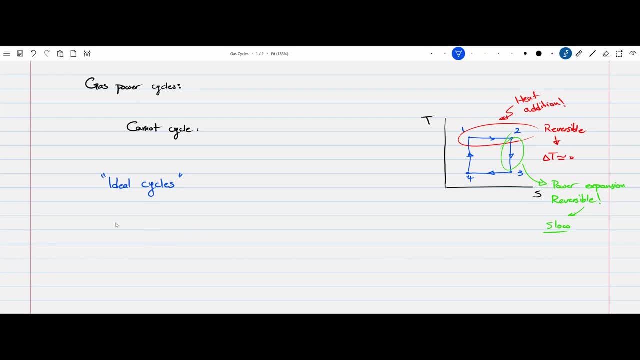 understand what is happening in a practical sense. So what makes the ideal cycle different from a Carnot cycle? For starters, we do not care for the processes to be truly reversible. We want them to be internally reversible. An internally reversible process means that we do care for the system to go back to its initial state. 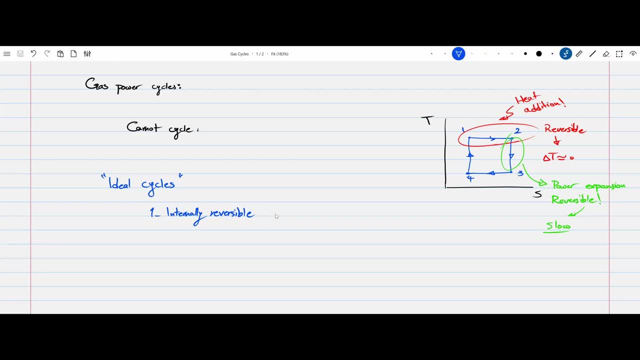 if we reverse the process but we do not care about the surroundings. So, for example, when we are adding heat, we want to make sure that the system can lose the same amount of heat and go back to its initial state, but we don't care what happens in the surroundings. 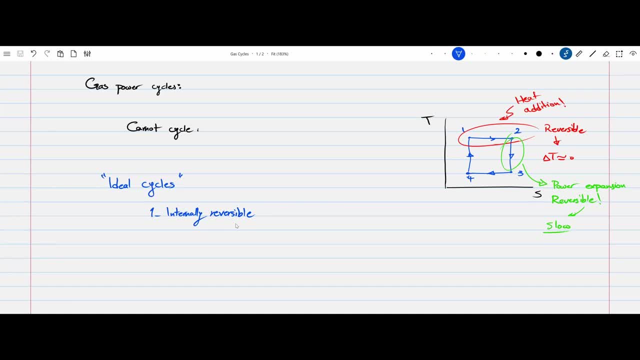 So that is the main difference between an ideal cycle and a Carnot cycle. These cycles are not reversible, they are internally reversible. So although the ideal cycle is now internally reversible, it is still an ideal cycle, meaning that we don't want to deal with any friction in. 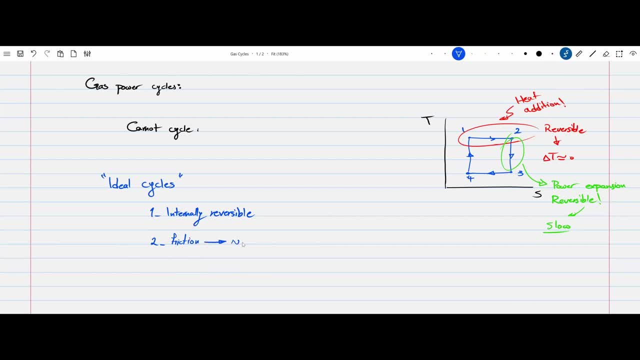 the system, which means no pressure drop In the system and also we don't want to deal with any unwanted heat transfer between the system and the surroundings. so no heat loss, And I want to emphasize unwanted heat loss. We are going to discuss gas cycles, ideal gas cycles, in this video. but even if you are dealing 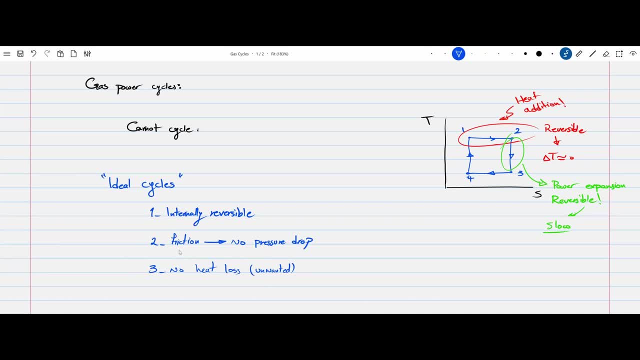 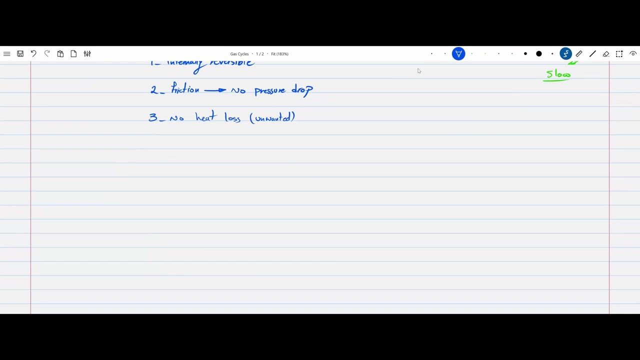 with ideal refrigeration cycles or ideal vapor power cycles. These three conditions are the same for any ideal cycle: It is internally reversible, There is no friction or pressure drop and there is no unwanted heat transfer between the surroundings. Now, focusing on the gas power cycles, we have to make a few assumptions regarding our working fluid. 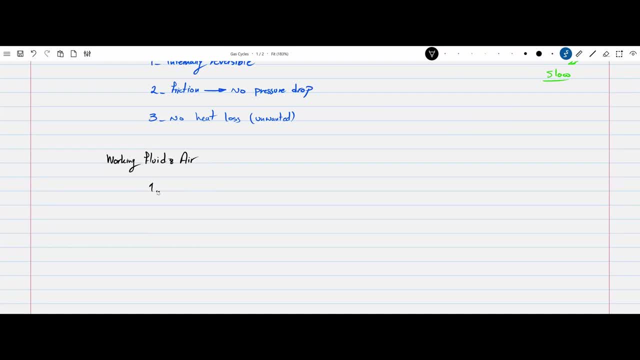 which is air. So the conditions that we are going to assume are very straightforward. Number one is that air is an ideal gas Throughout the cycle, regardless of what process it goes through. we are going to assume that air is an ideal gas. 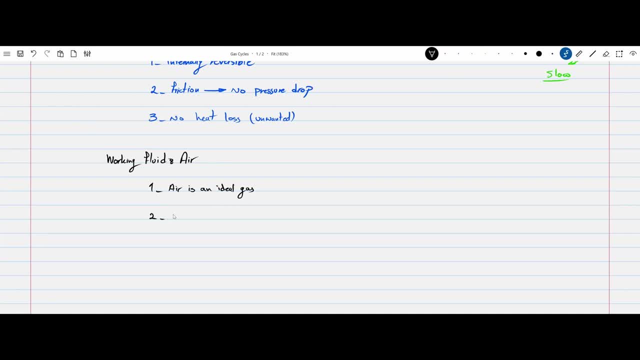 The second assumption that we make is that air does not leave the system or enter the system. Air is trapped in a closed loop. More on this later, when I'm going to show you how a typical cycle works. I'm going to explain why this is kind of true from a theoretical perspective and how it helps us analyze the cycles more efficiently. 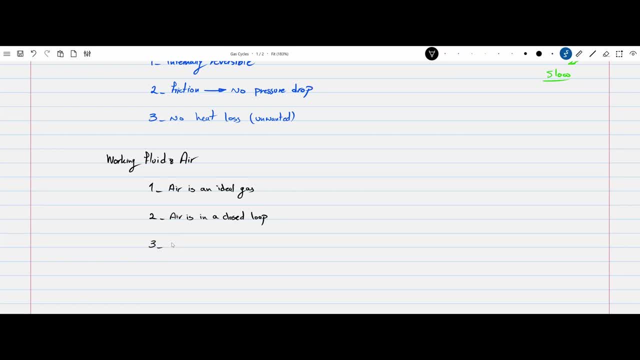 The next assumption that we are going to make is that the air composition through the processes is going to remain the same, Meaning that combustion, which we know in practice changes the composition of air, is not affecting air properties from a thermodynamic perspective. So, no chemical reactions. 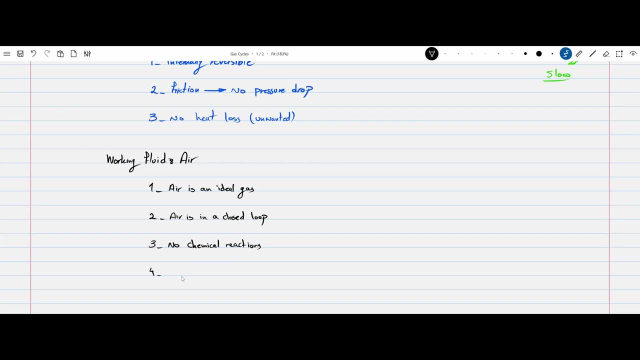 And finally, we are going to assume That the combustion, which is the source of energy in a power cycle, can be replaced by a heat addition process, And the exhaust process, where we, you know, push the combustion products out of the engine, can be replaced by a heat rejection process. 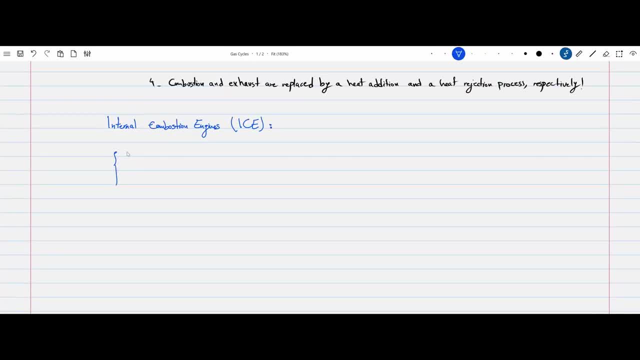 So internal combustion engines usually Fall into two categories: spark ignition And compression ignition. Now, the spark ignition engines are the ones that you see in your in your car. They usually run on gasoline, or just gas, as it is sometimes referred to. 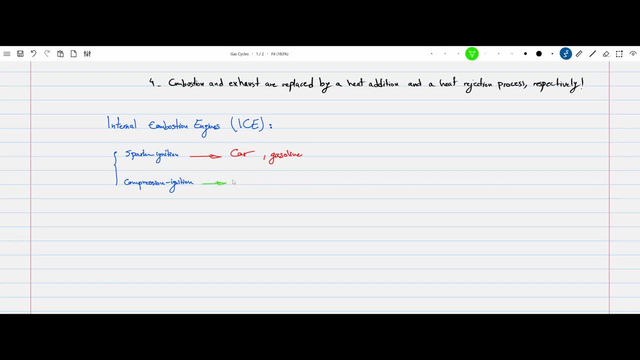 Compression ignition engines are the ones that we Usually have in more heavy-duty situations, like the ship propulsion or a tractor heavy machinery, And they are usually running on diesel fuel. You can have cars that are running on diesel fuel as well, which have the compression ignition. 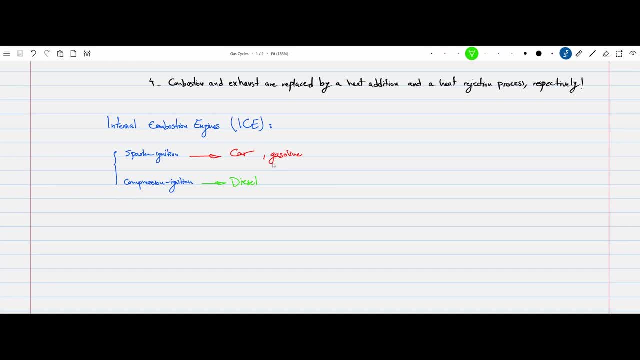 But most of the market is at least for commercial cars. But most of the market is at least for commercial cars, And the combustion engine is dominated by the gasoline Engines, which are spark ignition. Now, what is the difference between these two? 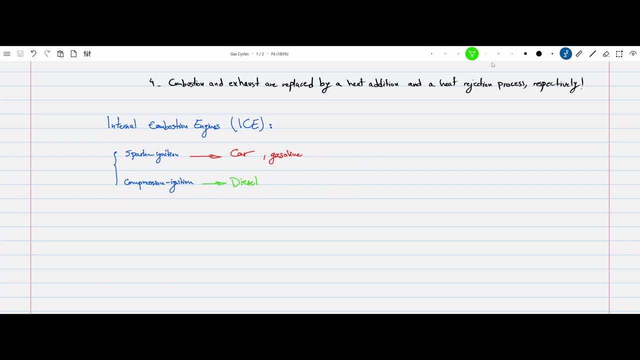 Before we go ahead with the cycles, it may be beneficial to discuss the differences. The difference is very, very simple, And the spark ignition engine relies on a external spark, if you will, To start the combustion process. You You may know that the cylinder in your car's engine has a component called spark, which 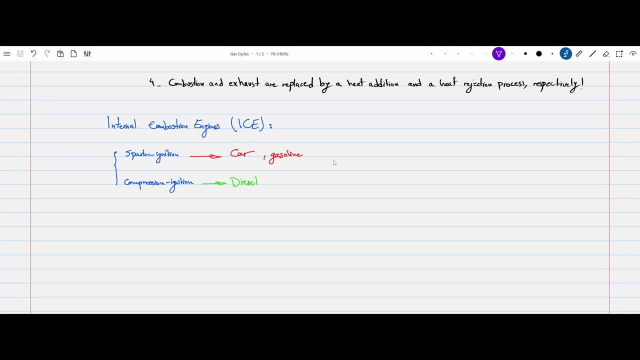 relies on electricity to create a electrical arc that starts the ignition of the gasoline inside your cylinder. So that's very easy to understand. Compression ignition, on the other hand, relies on the fact that some chemical components, When they reach a certain pressure or temperature, will start to ignite. 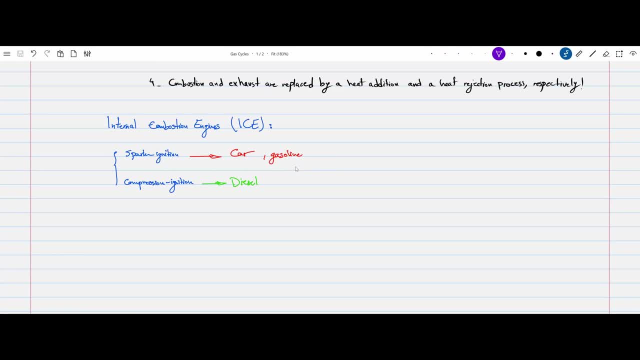 The ignition process automatically. That's how the compression engines work. They rely on the high temperature and high pressure of the gas mixture to start combusting on its own, and not rely on an external source like spark to start the process. OK, with that said, let's start talking about spark ignition engines. 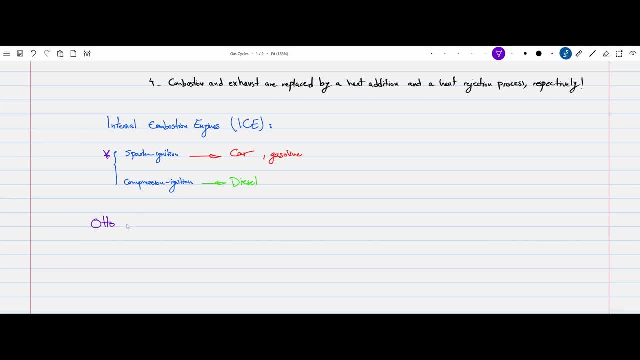 The cycle that Governs the spark ignition engine is called the auto cycle. Now here. I want to emphasize that in this video we are going to focus on a four stroke engine And not a two stroke engine. The principles are the same. 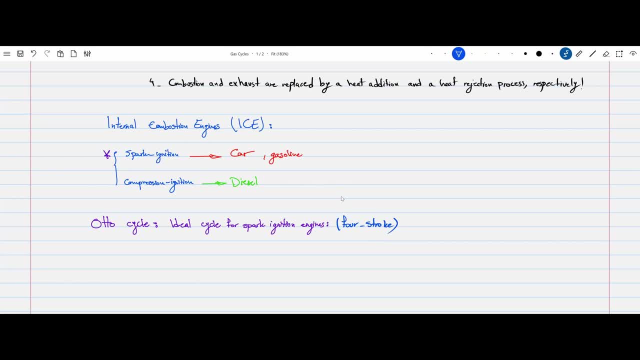 So probably you can do an analysis, if you really want to, on your own, But because the two stroke engines are of limited use, We are going to analyze the four stroke ones, which are the most common form of spark ignition engines. Now, before we can start talking about the actual process, we need to gather a bunch of information about an internal combustion engine. 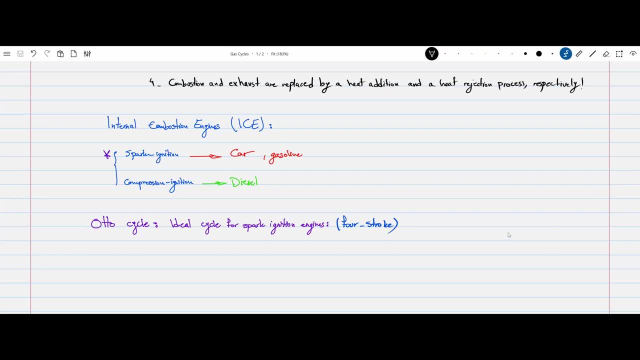 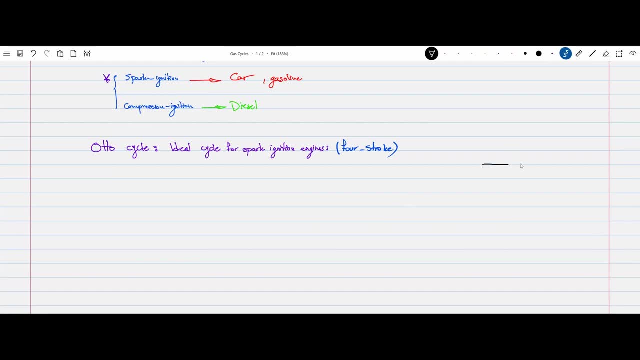 Mainly, we need to gather some information on the cylinder and the piston. So let's start. A typical piston and cylinder set up in an internal combustion engine looks roughly like this: Say, this is the cylinder And This here is the piston. 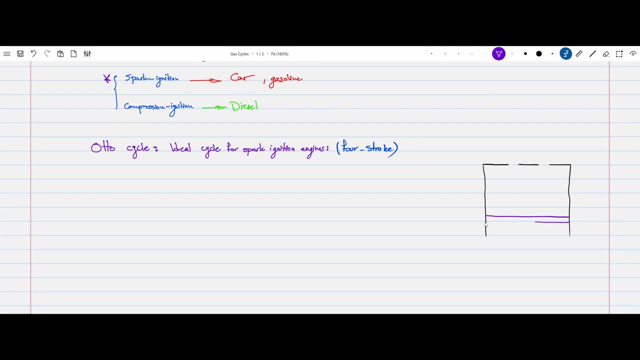 We have the intake valve And the exhaust valve on top of the cylinder, Like so. So this one is the intake valve And this one is the exhaust valve. Now the diameter of the cylinder usually is referred to as the bore of the cylinder. 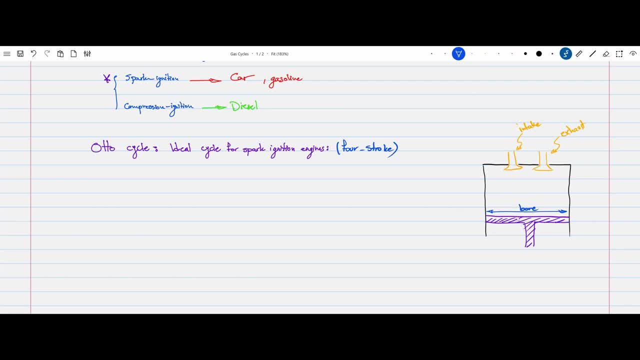 And there is a limit to the range of motion of the piston. What I mean by that is this piston can move up all the way to- maybe this point- It will not go all the way to hit this- The intake and exhaust valves. it can only move up all the way to the pink line. 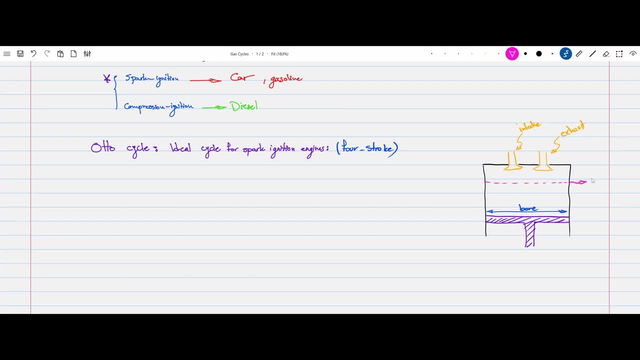 Now the pink line is referred to as top dead center. We show it with TDC And the volume above the TDC: the volume that the piston can move up and down. And the volume above the TDC: the volume that the piston can move up and down. 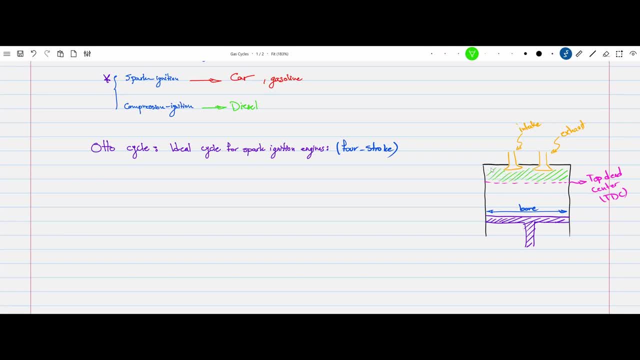 And the volume that the piston cannot touch is sometimes referred to as the clearance volume. So that much is clear. Nothing too crazy. We have the same limit on the bottom of the cylinder. The piston can only travel so much down inside the cylinder. 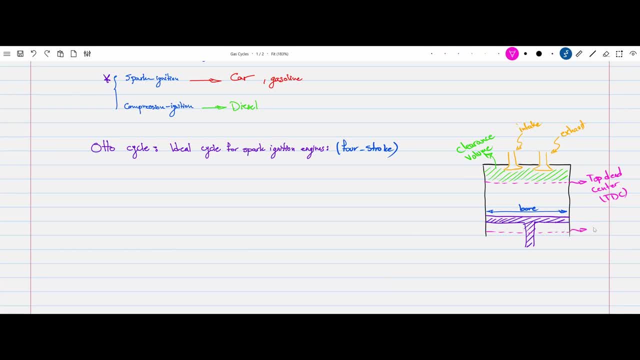 Let's say that's the pink line again on the bottom. We call this the bottom Bottom dead center And we show it with BDC. Now the length of a single stroke of the piston is the distance between the two dead centers. 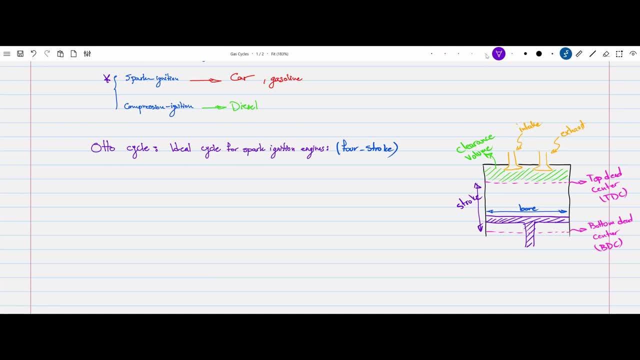 And the volume in between, the volume between the TDC and the BDC is referred to as displacement, And the volume in between, the volume between the two dead centers, is referred to as displacement. So when you check your car's engine and it says, for example, a 2.4 liters or something like that as the capacity for the engine, 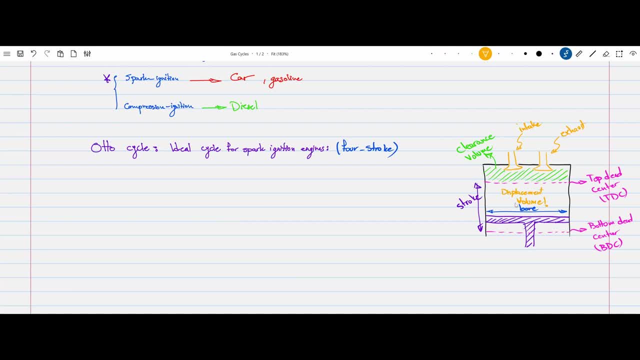 it is referring to the displacement volume of each of the cylinders in your engine. Your car engine typically has something between four to eight cylinders, depending on the model make and how loud you want the engine to be. Okay, so, based on this little drawing here, we can introduce a very important 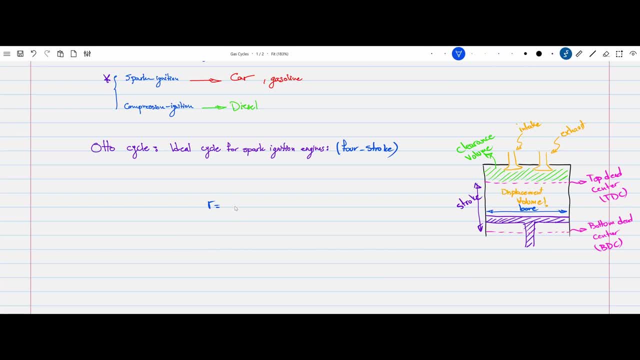 physical property of an internal combustion engine. We show it with R and it is the ratio of the maximum volume to the minimum volume within our system. Now, if we look at the drawing, the maximum volume for our system is the volume of the system when the piston is at the very bottom. 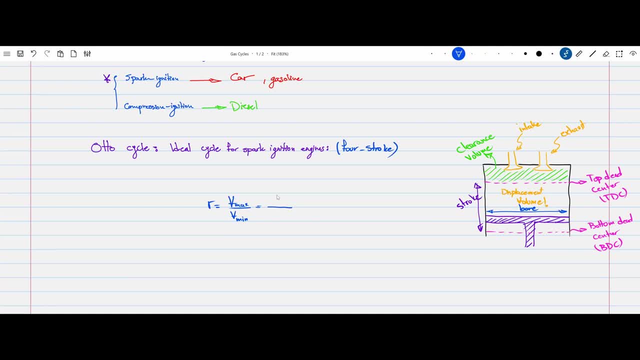 So one can make the argument that this is the volume of the bottom dead center. With the same logic you can see that the minimum volume for your system is when the piston is on the very top, which is the top dead center. and you can say the V minimum is Tdc or also the clearance volume. They would be the same thing. 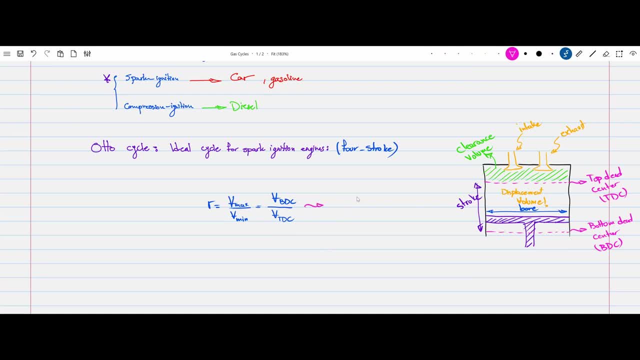 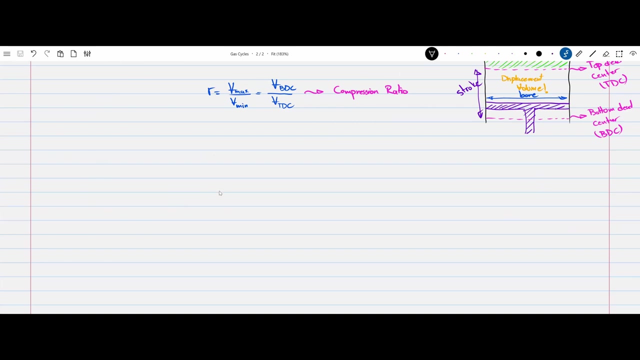 We refer to this property as compression ratio. This is very important, and we are going to see this later within the equations that we are going to drive for the auto cycle. Okay, now let's see if we can develop an idea of how a four-stroke engine actually works. 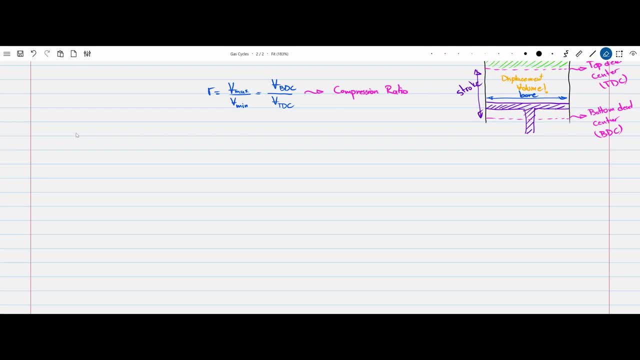 Overall, there are different ways of looking at the sequence of a four-stroke engine. For me personally, I like to start from where the fresh mix of air and fuel- air and fuel- enters the cylinder. So we are looking at the scenario where the piston is at the top of the cylinder here. 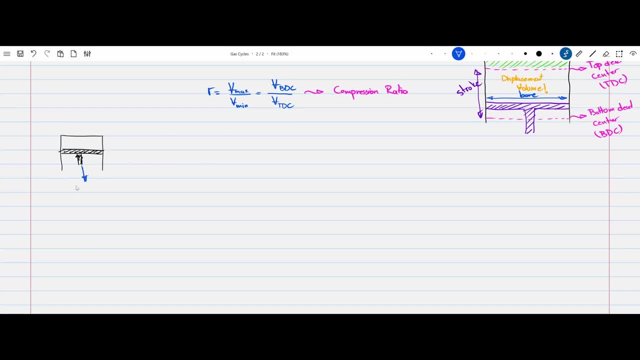 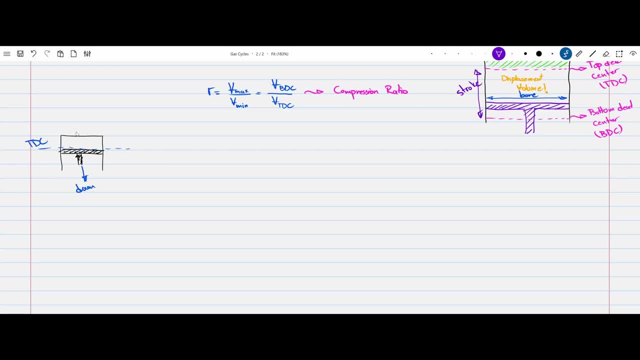 So, while the piston moves down, the volume in the piston expands and a fresh mix of air and fuel enters the cylinder. Now please take note that this expansion of the piston down and entrance of the fuel into the system makes the system experience a constant pressure expansion. 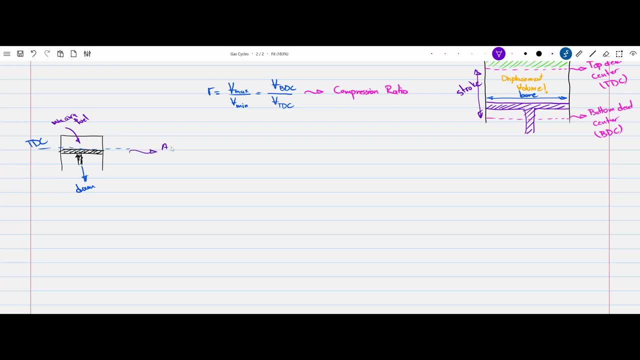 So this can be approximated by a constant pressure process. I would like to show this process on a diagram with zero to one notation. I'm going to keep track of what is going on on this PV diagram. So this is R and this is volume. 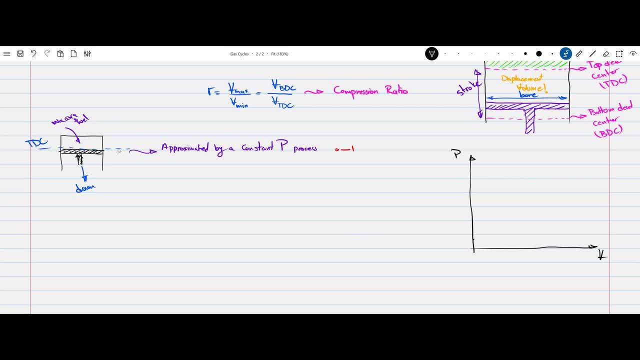 Now the thing about the mixture of air and fuel is that typically you are looking at an air mixture that is entered the engine from the grill in front of the car And usually you are looking at the air at atmospheric pressure. So I'm going to say that process zero to one is going to change. 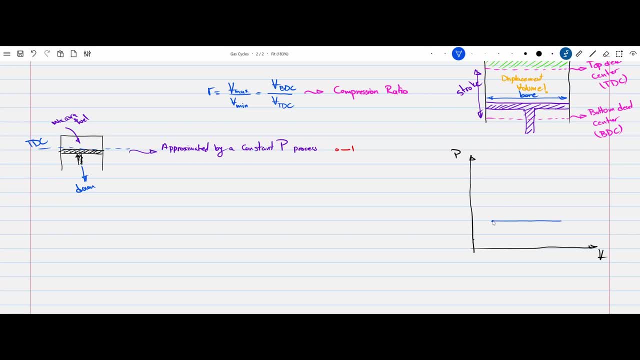 So I'm going to say that process zero to one prevents the received voice from entering the engine and the car, So parents have to be, and parents have to be, So parents have to be. one looks like this kind of keep in mind. we are looking at the practical problem right right now. 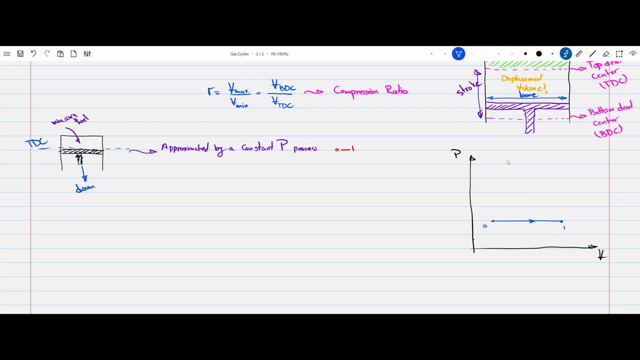 so this is zero to one. a few things that are worth mentioning is that, remember, the process starts where the piston is at the tdc, at the minimum volume, so this is the minimum, and the process ends when the piston reaches the bdc, the maximum volume. so right away you can see that the maximum volume in our system is equal. 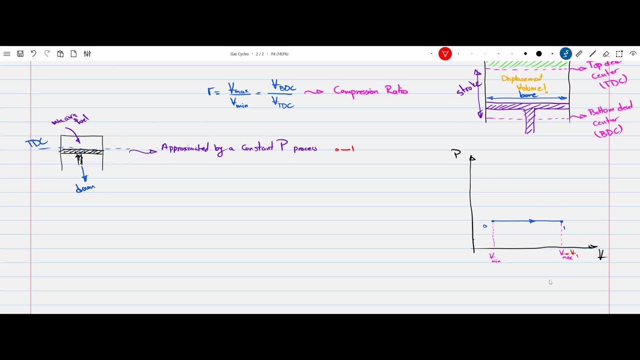 to the volume of state one now. keep that in mind and we are going to continue. so the next process begins right here. right after, when the piston hits the bdc, the piston starts to go up again. it will be the second stroke, right. the piston starts to move up, during which both the intake 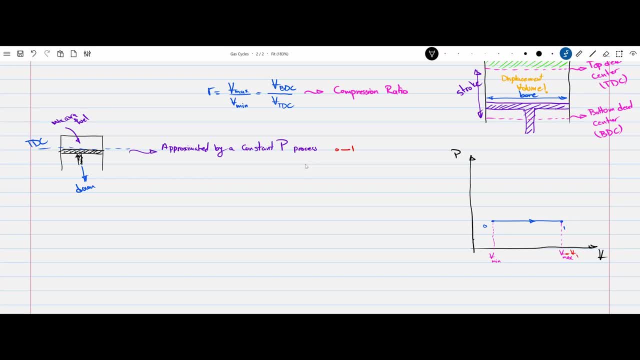 and exhaust valves are closed and this air mixture is going to get compressed. so the second process: the piston was all the way down. now it's moving up from the bottom, that center. now both intake and exhaust valves are closed, so we are going to experience compression. so this compression, 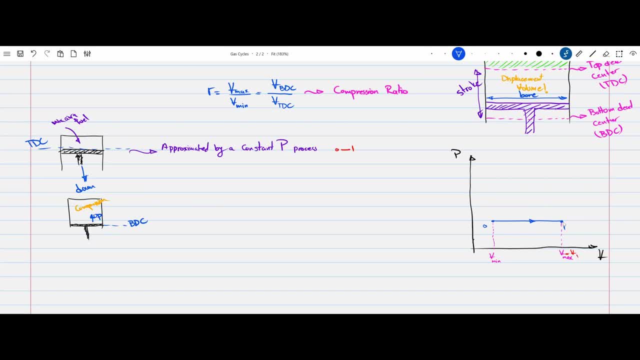 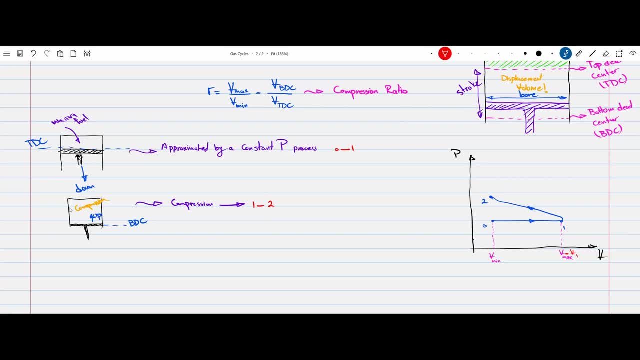 where you get one, two, two. now please keep in mind that the piston, while going through the compression, can only reach to the tdC right. so the volume of the system. And that's where you get one to two. Now please keep in mind that the piston, while going, 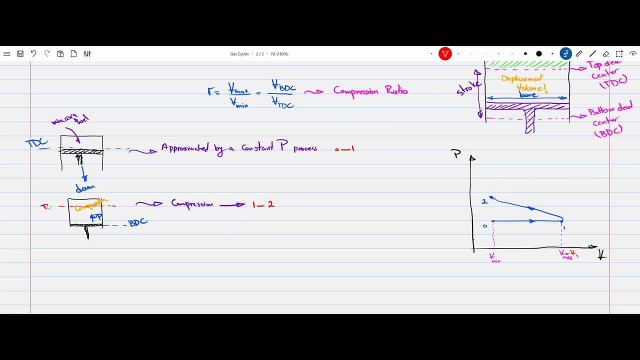 through the compression can only reach to the tdC right. So the volume of the system at state 2 is equal to the minimum volume, which for some reason isn't gonna mean bad enough. instantly tells me that the minimum volume of the system is equal to volume 2. 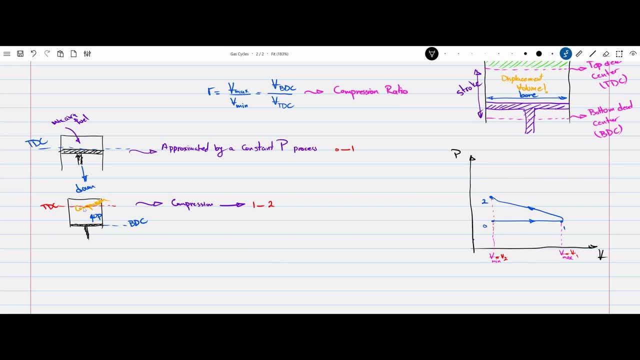 the moment the piston reaches the top dead center, something very interesting happens. the moment that the gas is compressed to its fullest, the spark ignites. the mixture, now this combustion, so this is the spark. it happens so fast that the piston has not yet got the chance to move down. 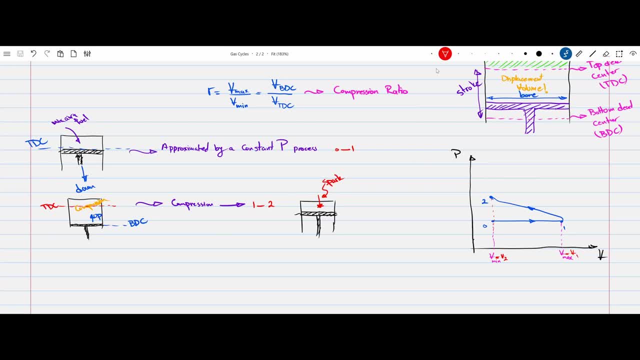 when the burning process is happening. so this burning process, or combustion process, is the process that, with our assumptions we mentioned. we are not going to go through the chemical reaction, but we are going to model it as a heat addition, right? so first of all, I would like to show this heat addition. 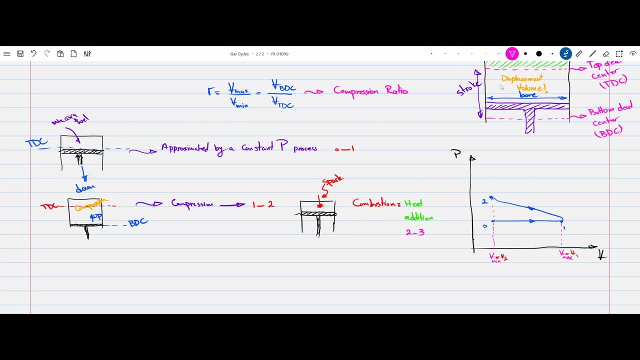 process with 2 to 3 notation. so now I can show this combustion with a process 2 to 3 like this. keep in mind that the piston has not yet have chance to start moving downwards. so the whole heat addition part or the combustion part. 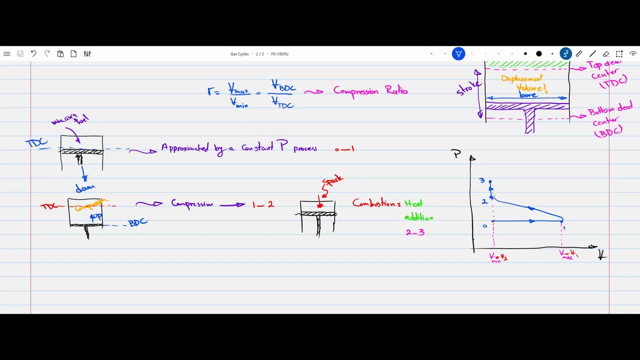 happens at the constant volume from 2 to 3. next on the stroke list, the hot gas here, because of the combustion, is now experiencing high pressure. you can even see that here when we added heat or the combustion process from 2 to 3 while the piston was on. 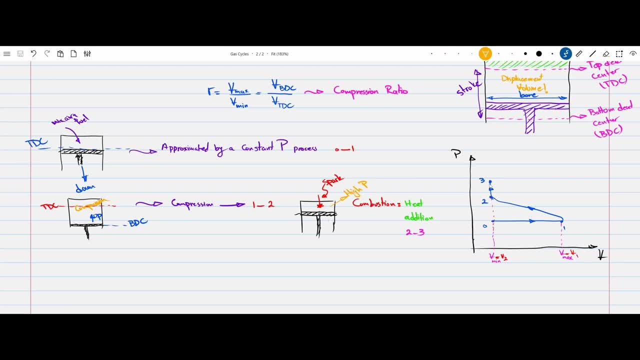 top at the TDC, the pressure of the gas spiked high right. so this high pressure gas is now pushing the piston down. so for our next stroke, we have a scenario where the piston is moving downwards due to the push by the high pressure gas, and this is the. 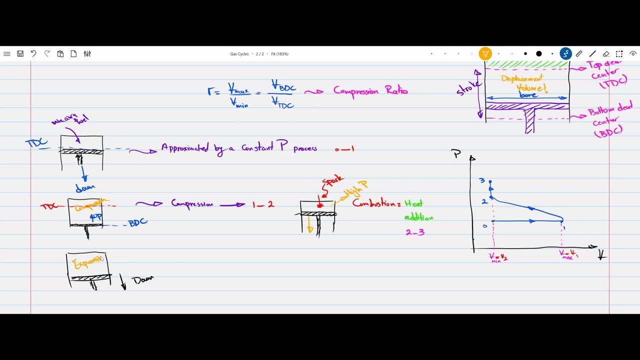 in other words, this is an expansion. so the third stroke is the expansion due to combustion. I would like to show this with 3 to 4 notation on the PV diagram. so from 3 to 4, you're expecting to see something that looks like this: 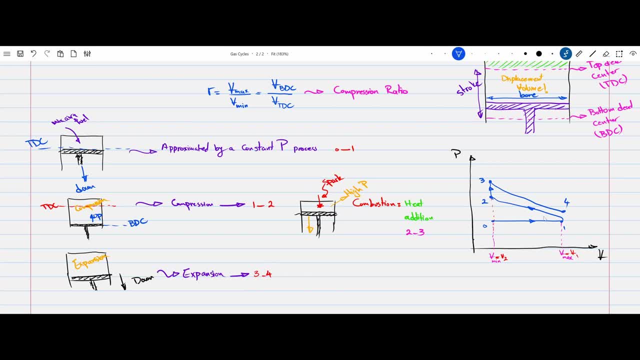 now please keep in mind that this piston can move to a certain range. it can only move all the way to bottom dead center and, as we discussed in the first stroke, we know that the bottom dead center is volume 1. so you can kind of see that volume 4 is equal to volume 1. 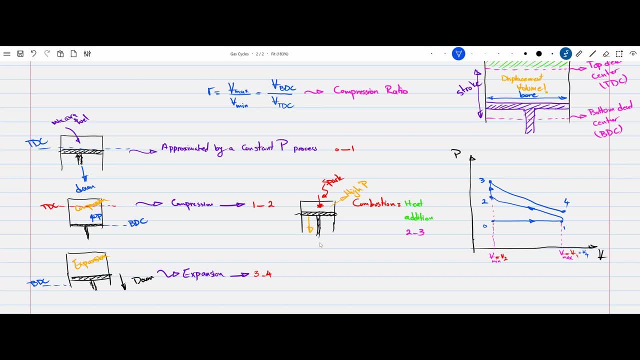 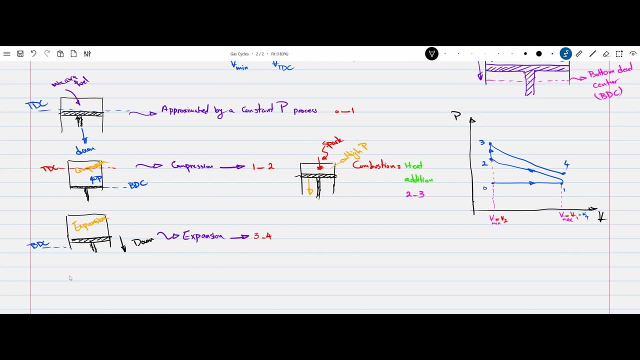 because it's the bottom dead center. now, finally, for the last stroke, we have the piston moving up again due to the rotation of the crankshaft. this time, when the piston is moving up, it is pushing out the burnt mixture of air and fuel and it's moving up the piston. 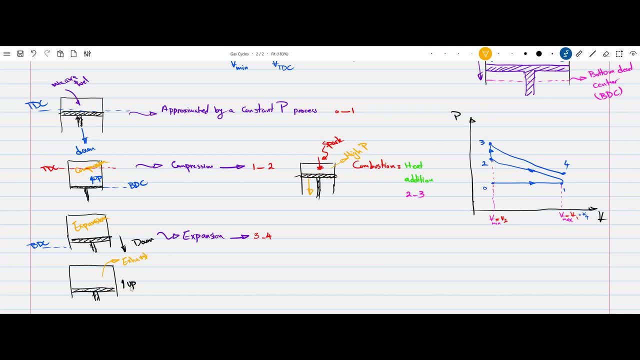 through through the exhaust valve, because the piston is moving up and the gas is moving gradually out of the system, we can kind of assume that the pressure within the system remains constant. so this is the fourth stroke and I would like to show it with process 4 to 0. 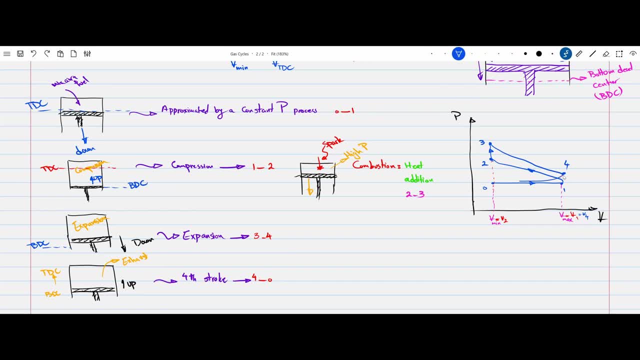 now, as I said, the pressure remains constant for this process where the burnt air gas mixture is leaving the system. so now you have all four strokes of an engine. the next stroke now that the piston is on the top dead center. the next stroke is the first one that we had here. 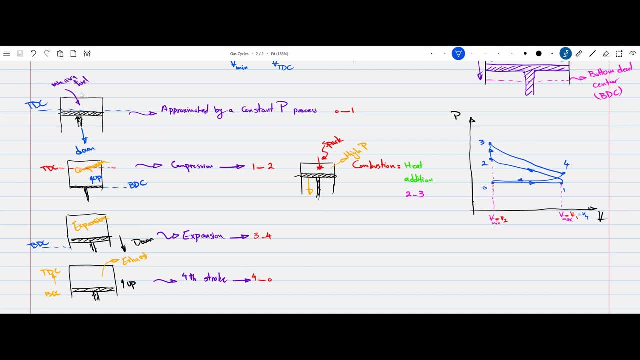 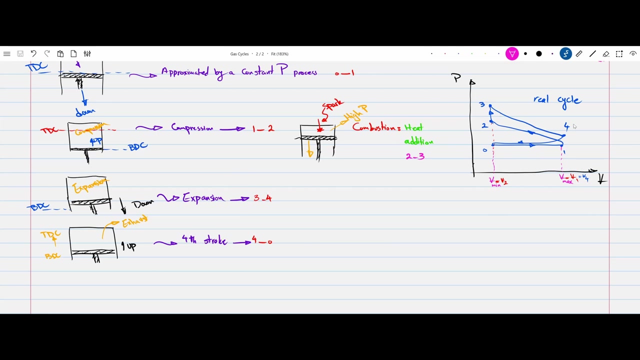 the piston starts to go down, mixed air and fuel will enter and the cycle starts again. so these are the four strokes and this diagram here is the practical or real cycle that the air goes through. now, through the analysis of four strokes of an internal combustion engine, we were able to come up with the real cycle pv diagram. 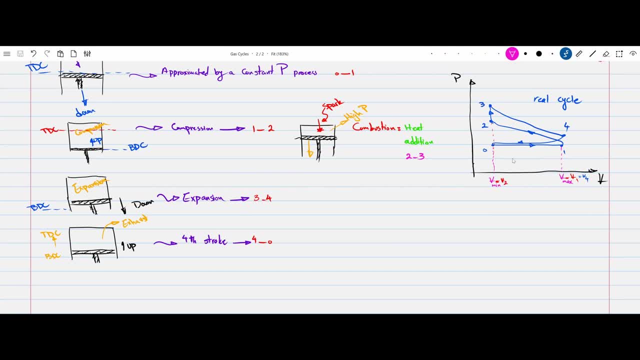 but we are far from an ideal cycle here. first of all, if you review the assumptions, we want to treat air as a working fluid that is trapped within the system. from a practical, real point of view, the air that enters your engine and goes through the four strokes leaves through the 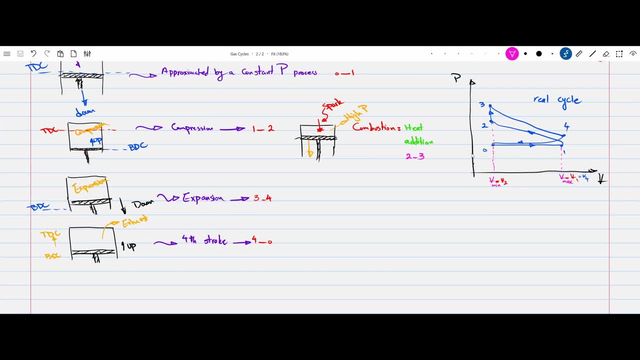 exhaust and goes out of your car. right, that is you. So one's process will not prevent the process from four to zero. however, from a thermodynamic analysis perspective, we really don't want to lose that air out. so let's take a closer look at processes zero to one and process four to zero. 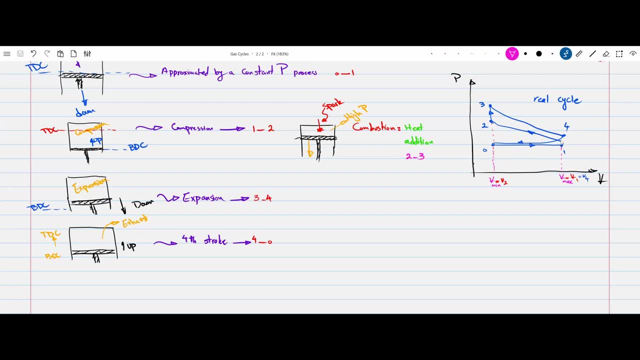 one can make the argument that zero to one and four to zero are very, very close to each other in opposite directions. so if, for example, you are MyQubroken, Air sets the shirt off. here one works with maneuverable airchecks and they add an option to it which is dead heavy to one on top of this in the other direction, in case you happen to need support to get it out of the airdie. air in both a straight line. if you have any variation in the middle, it does your job to expand into different directions. 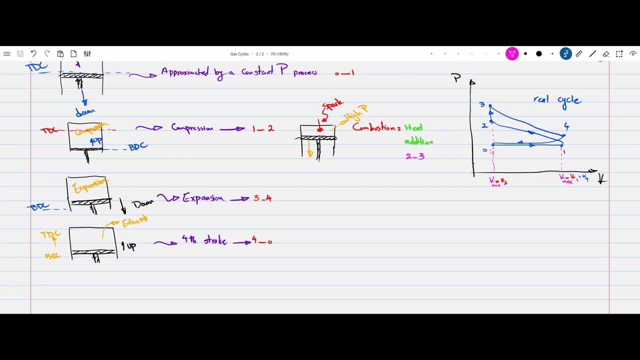 Analyzing this from a work perspective, 0 to 1 is an expansion, So you are getting some work out of this expansion. Whatever the work is, that will be equal to the area of the pink shaded rectangle From 4 to 0 perspective. you are looking at a compression. 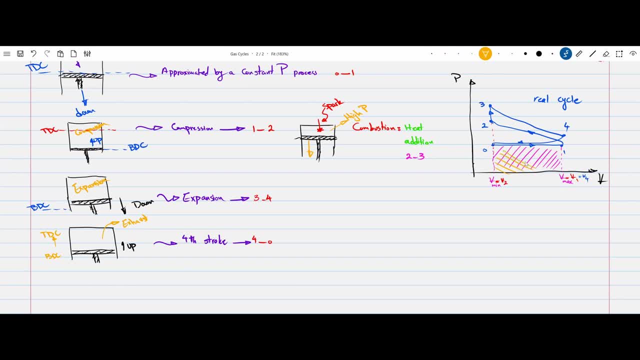 So from 4 to 0, you are applying work to your system to compress the air out of the cylinder, And that amount of work is the orange rectangle. So you can see that the orange and the pink rectangles are kind of the same. 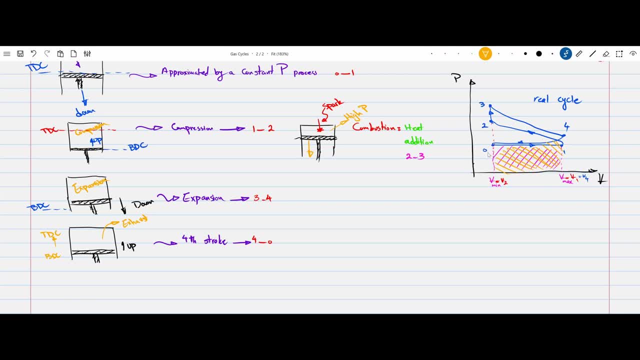 Indicating that whatever work you are getting from 0 to 1 is equal to whatever work you are losing from 4 to 0.. If we focus on the heat addition part 2 to 3, you can clearly see that this heat addition is a constant volume process. 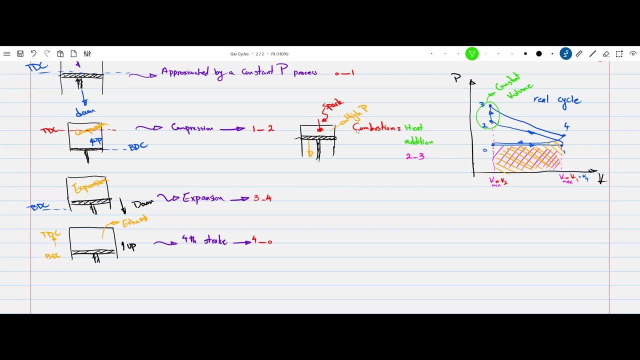 If you track the volumes down, you see that the entire combustion happens when the piston is at TDC, which is the minimum volume of our system, as you can see down here, And so 2 to 3 is a constant volume process. 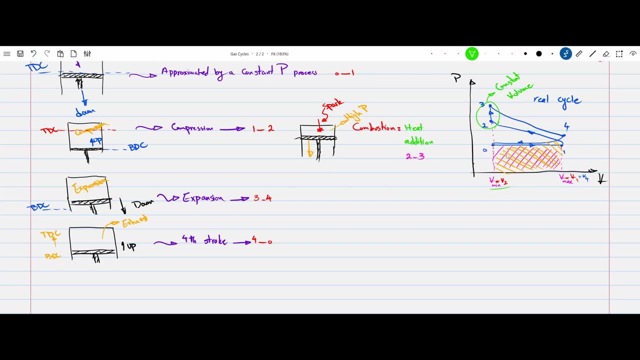 Now that we know 4 to 0 and 0 to 1 are kind of the same processes, we can look at 4 to 1.. Yes, in a real cycle they are not connected, But when you look at 4 and 1, you realize that they are sharing the same volumes at states 1 and 4.. 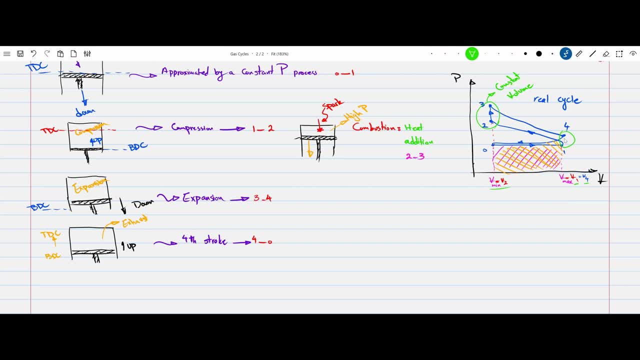 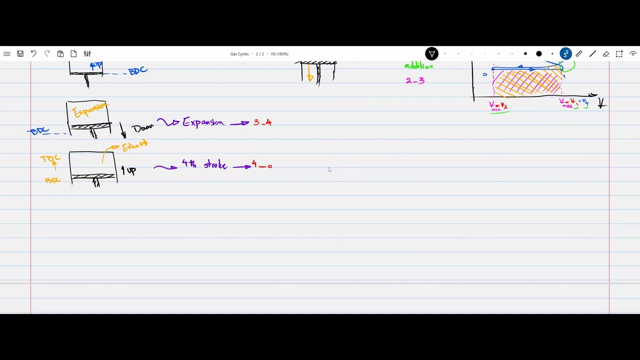 And 4 to 0 and 0 to 1 are the same. So it kind of makes sense to treat this portion of the cycle As the heat rejection parts and replace it by a constant volume process. If we do that then we can come up with the PV diagram of an ideal Odo cycle. 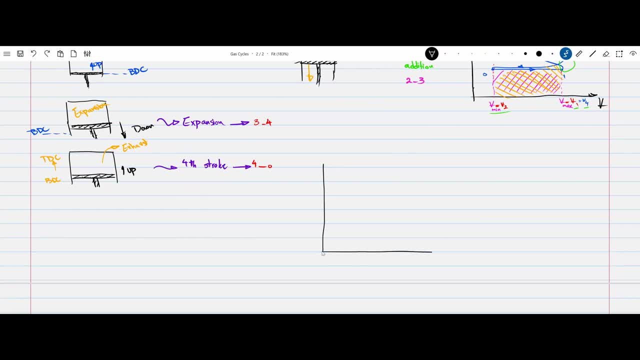 So let me draw it down here for you. So this is P. this is volume 0 to 1,, 1 to 2,, 2 to 3,, 3 to 4, and 4 to 1.. Putting the small arrows just to show where the cycle moves. 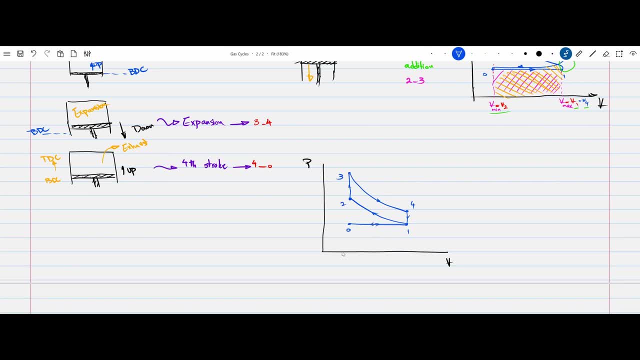 0 to 1 and 1 to 0.. So this is the ideal Odo cycle. In this ideal form, 0 to 1 and 1 to 0 are constant pressures. 1 to 2 is an isentropic compression. 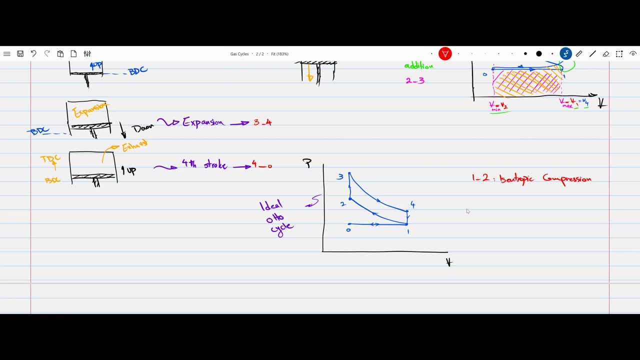 1 to 2 is an isentropic compression And 1 to 1 is an isentropic expansion And 1 to 2 is an isentropic expansion. 2 to 3 is a constant volume heat addition. 2 to 3 is a constant volume heat addition. 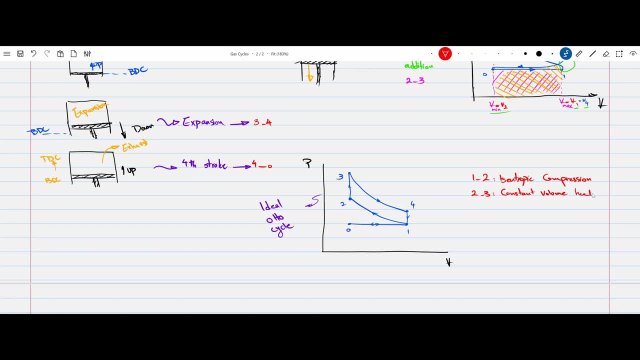 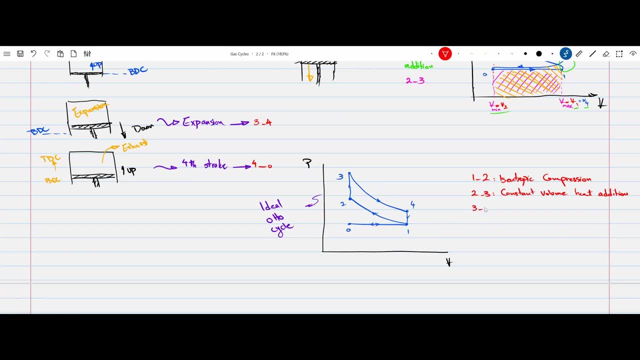 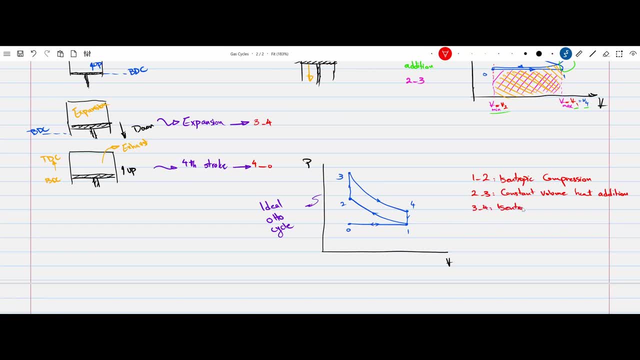 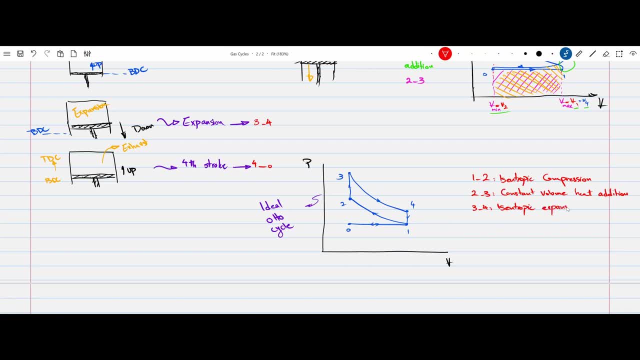 and 4 to 1 is a constant volume heat rejection. okay, so why we are saying isentropic compression and isentropic expansion? we did not cover that in the practical, real cycle for understanding these two processes- the isentropic compression, isentropic expansion- we need to go back to the assumptions that we made at the beginning of the 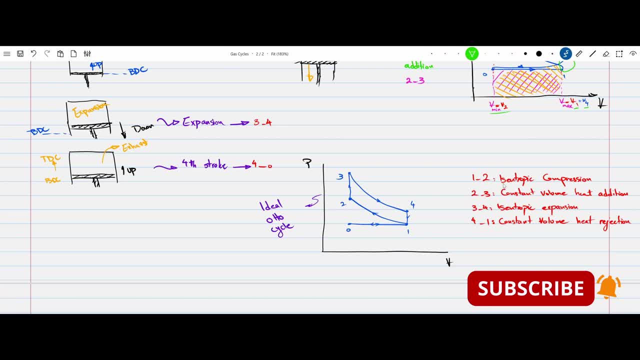 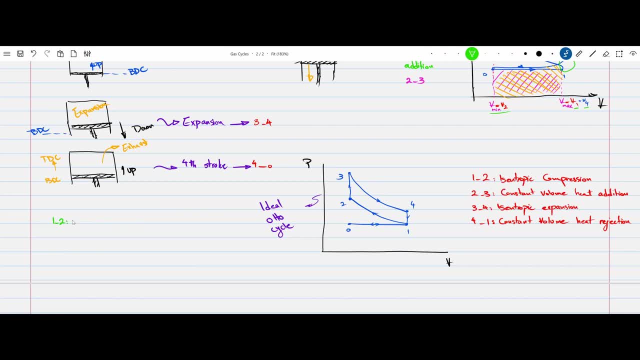 now look at the process 1 to 2. if 1 to 2 is frictionless and also is not experiencing any unwanted heat transfer, in other words, is adiabatic, then it is isentropic. right, that's what it is. this is an isentropic process. the same goes for 3 to 4. 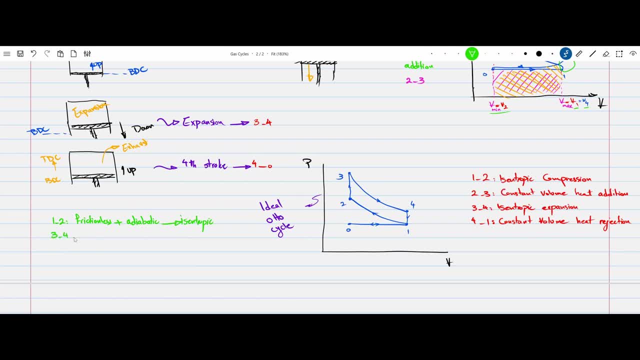 it is frictionless. right, that's what it is. 3 to 4: it is frictionless and it does not have any unwanted heat transfer, meaning that it is also adiabatic, and so it is also isentropic. isentropic, so for an ideal cycle- auto cycle- we are dealing with 2 isentropic processes and 2 constant volume processes. 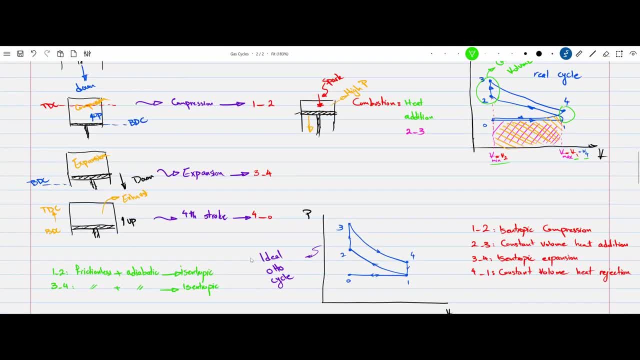 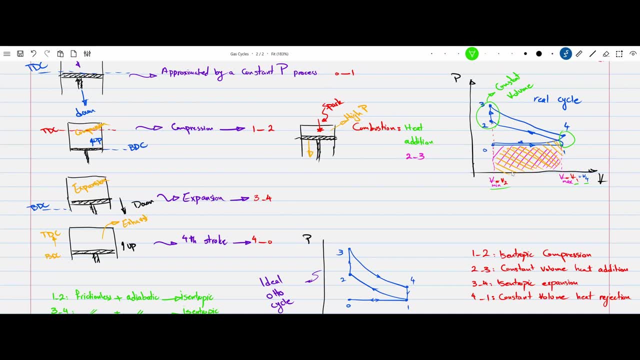 again, as you can see, let me scroll up a little bit, as you can see again, as you can see, let me scroll up a little bit, as you can see, the ideal and the real. they are not a hundred percent match, but the ideal, through these assumptions that we made, is a good approximation on what is actually happening within the real. 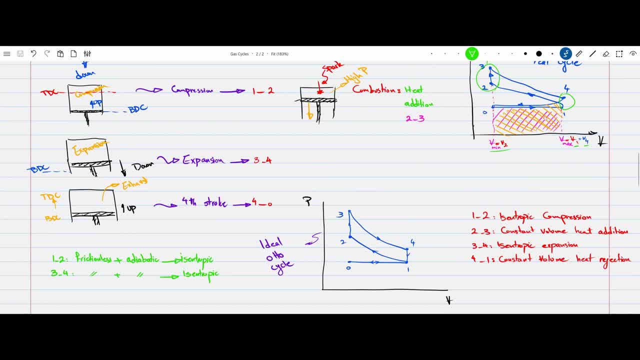 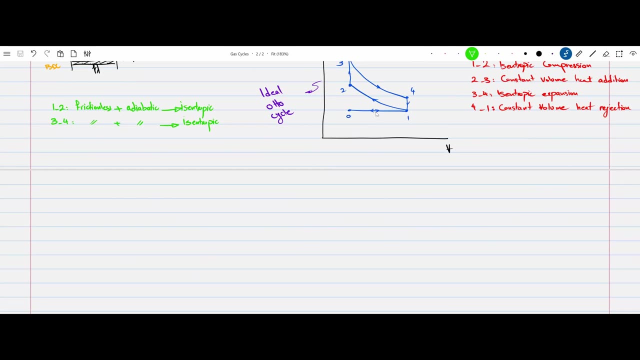 cycle. now, based on the orange and pink argument that i had for the work uh done and the work required for processes zero to one and one to zero, we can see that this line on the pv diagram is not that important and in most references and in most applications, like 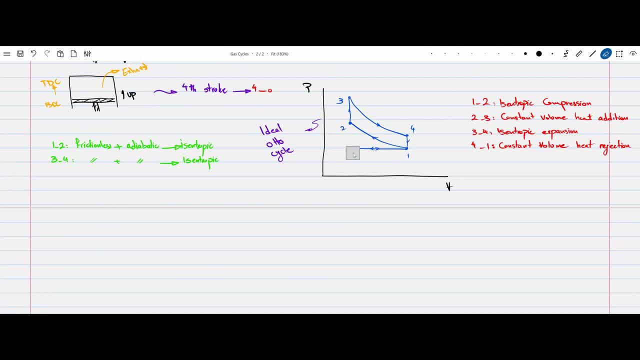 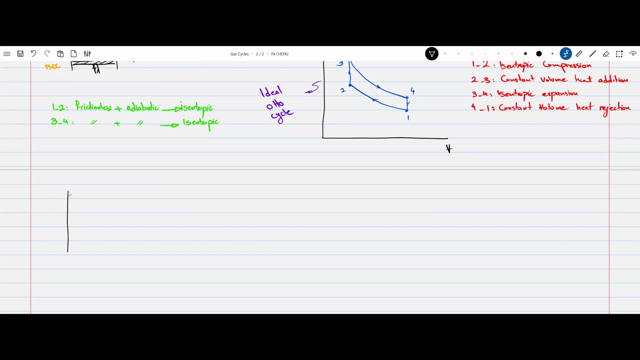 99 of all the applications. this line is not even shown. this one, two, two, two, two, three, three, two, four and four to one is the ideal auto cycle. we can add the ts diagram to this analysis as well. so let's say this is t and this is s. the processes are very simple. 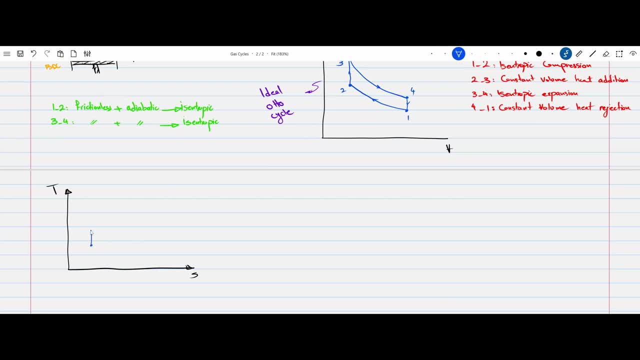 one to two is a isentropic expansion, so s is not changing. two to three is a heat addition at constant volume, so you're looking at something like this: three to four is again an isentropic expansion, so s does not change, and four to one is a constant volume. 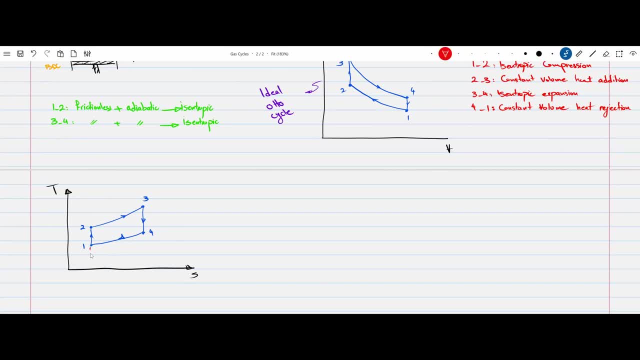 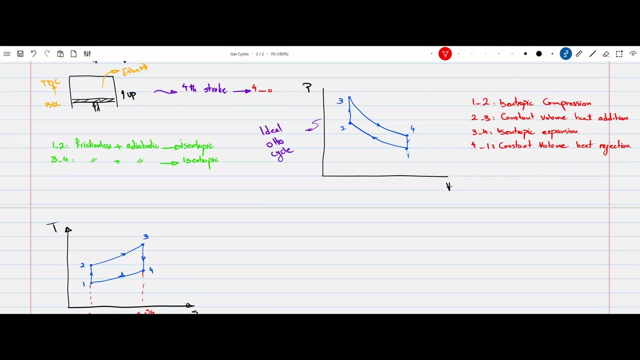 heat rejection. so please take note that in this diagram s1 and s2 are the same. s3 and s4 are the same. on the previous diagram also, please take note that v1 and v4 are the same, whereas volume two and volume three are the same. 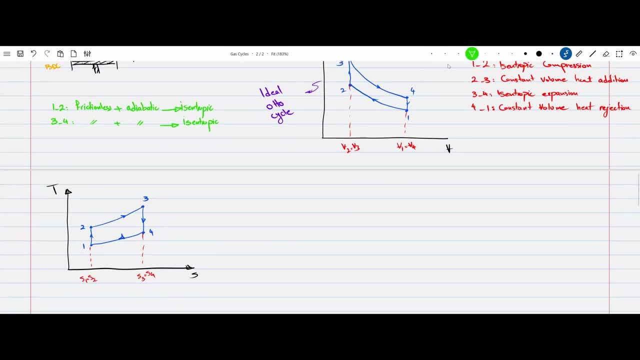 all right. so two to three is the heat addition, whatever heat right here. so havia one is gradually increasing and you can see that what's happening here is that we've got sur cube v0 equal to one over and rate, and here we'll just take a times comparing it with the thermal dynamic notation that we have. 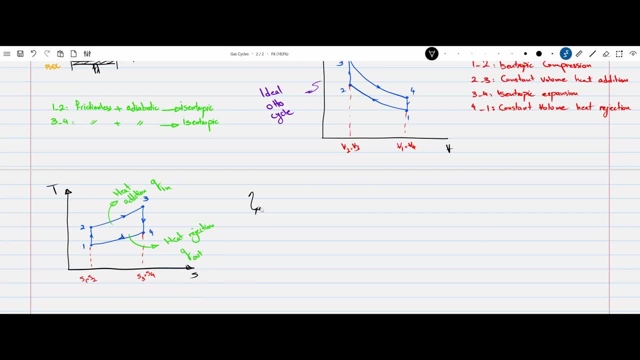 this is where q in happens. four-to-one is heat rejection or with thermal dynamic notation. this is q out, this one minus Q out over Q in for each of the processes. for each of the processes on this diagram. we know that the first law of thermodynamics holds. 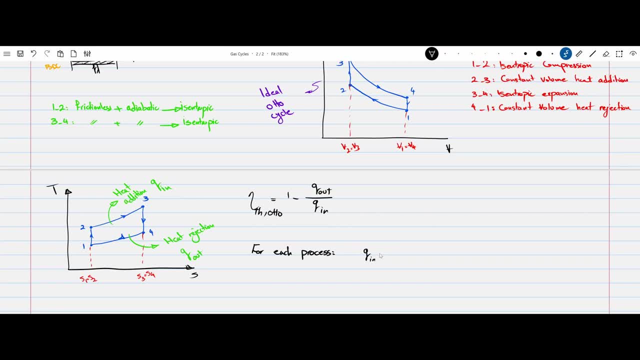 true. so Q in minus, Q out, plus. work in minus, work out is the change of internal energy. you might have noticed that I'm using small letter notation. Q's works and you, because if this is a closed system, which we know, it is based on our assumptions. the mass in the system is: 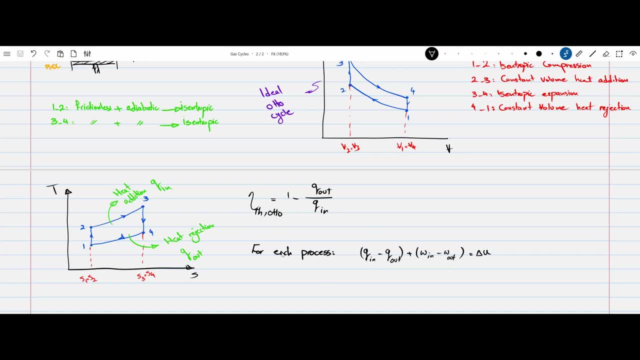 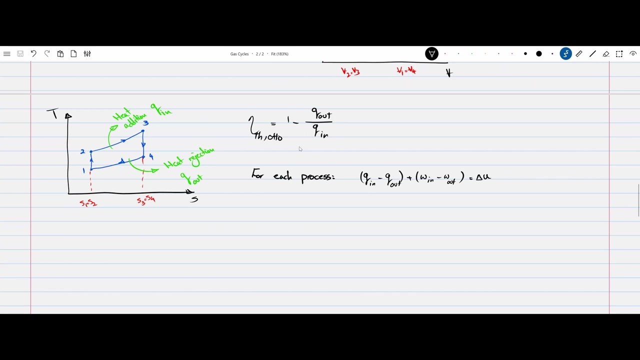 the same. there is no mass entering or leaving the theoretical cycle, so I can divide everything by the mass of the system and work with the per mass intensive units. okay, so with that out of the mind, out of the way, let's focus on what you want to do. I want to calculate the thermal 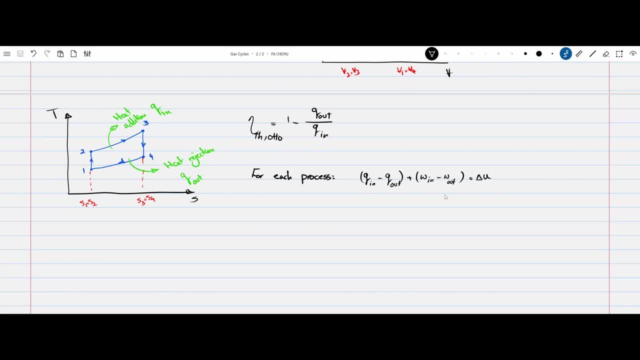 efficiency of the system and I want to calculate the thermal efficiency of the system. and I want to calculate the thermal efficiency of the system and I, this cycle and for each process, the first law of thermodynamics is true. from the thermal efficiency equation I can say this is actually Q from process 4. 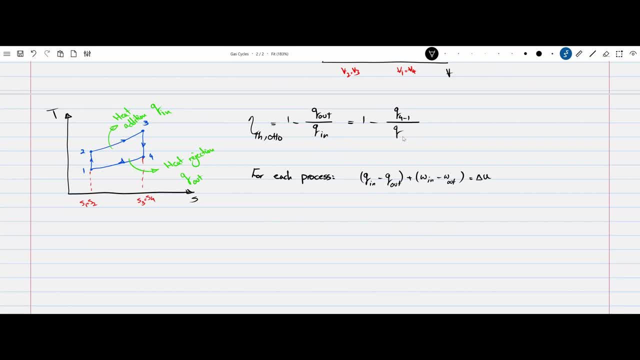 to 1 over the Q for process 2 to 3. so these are the two processes that I need to focus on, starting with the process 2 to 3. So this is a constant volume process. So because the volume is constant, the boundary work is non-existent, right. 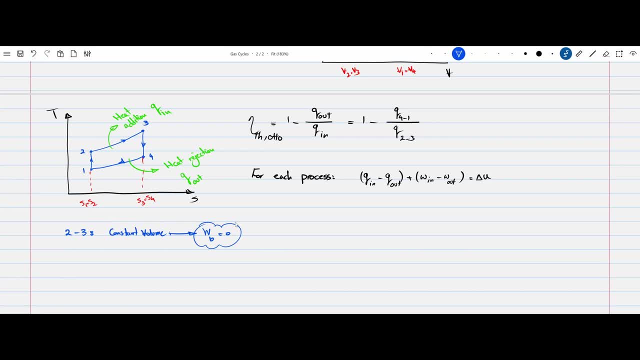 We know that there are no other forms of work available here. There is no electricity, there is no shaft moving, nothing except the boundary work. So there is no work in and out for the process 2 to 3.. Therefore the first law of thermodynamics says that the Q in for the process 2 to 3 is internal energy at 0.3 minus internal energy at 0.2.. 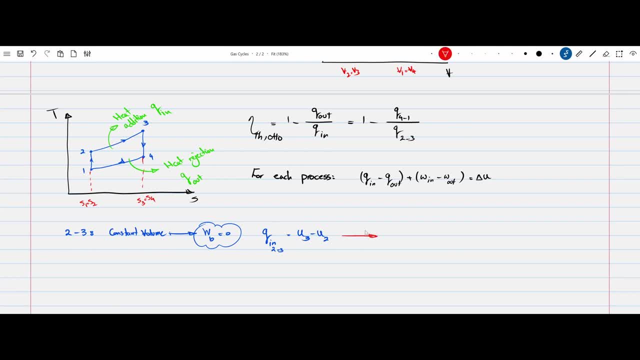 Now for an ideal gas. we know that the change in internal energy can be approximated by CvT3 minus T2. So I have the Q in the process 2 to 3.. Now let's focus on the process 2 to 3.. 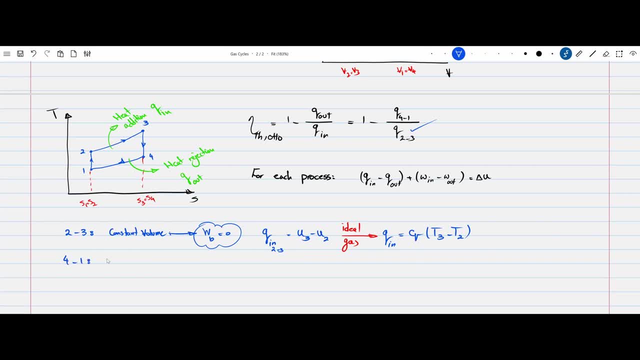 Now let's focus on the process 4 to 1.. This is again a constant volume process, Meaning again there is no boundary work available. Again the Q based on the first law of thermodynamics that I've written above. 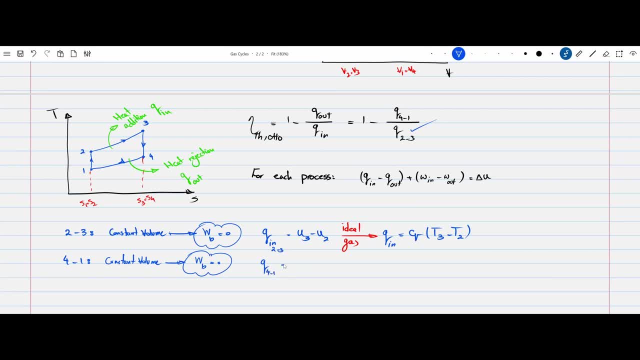 the Q from 4 to 1, is going is going to be simply U4 minus U1.. For an ideal gas, again, the change of internal energy can be approximated by CvT4 minus T1.. So now I have the Q from 4 to 1 as well. 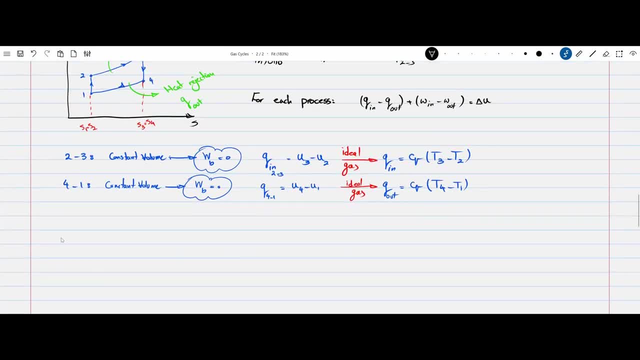 Let's set this up here Again. so the thermal efficiency of an otocycle is 1 minus Q out over Q, in which is 1 minus CvT4 minus T1 over CvT3 minus T2.. Cvs cancel each other. 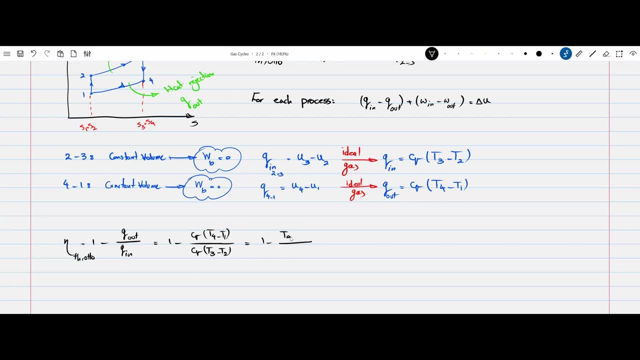 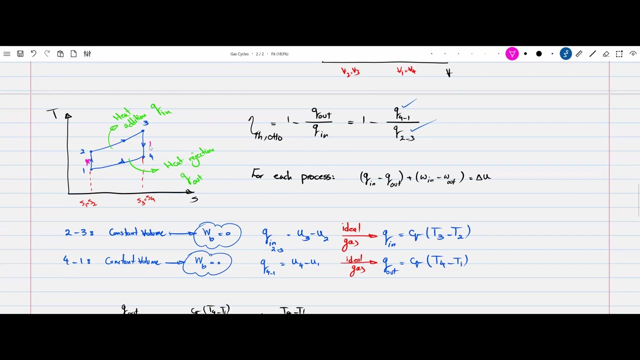 And you end up with 1 minus T4 minus T1, over T3 minus T2.. Okay, so let's keep it here for the time being And let's now focus on the other two processes that we kind of neglected: Processes 1 to 2 and 3 to 4.. 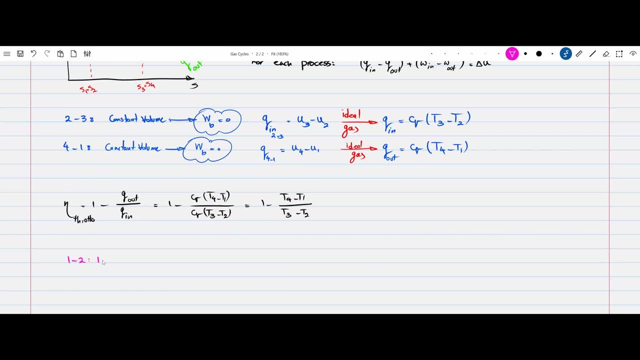 Starting with 1 to 2, it is an isentropic process. We know that, for an isentropic process, T1 over T2 is equal to volume 2 over volume 1 raised to K minus 1.. K being the ratio of specific heats. 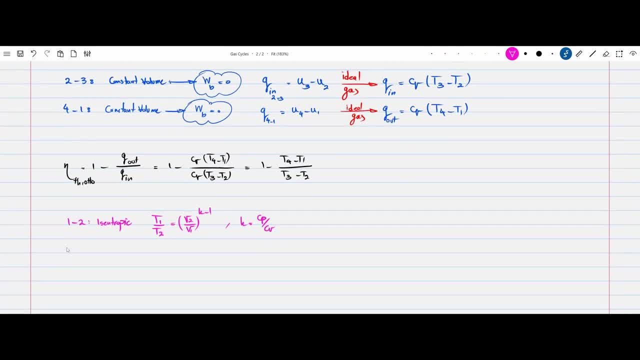 For the other process, process 3 to 4, we have again an isentropic expansion right. So on these isentropic expansion, again, one can use the isentropic equations for an ideal gas: T4 over T3 is V3 over V4 raised to K minus 1.. 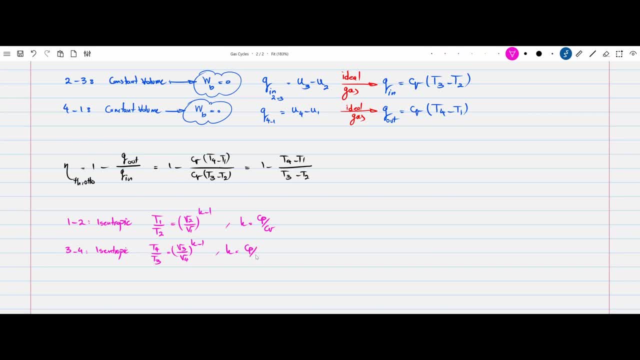 K being the same thing, Cp over Cv, specific heat ratio. Now please take note that because 2 to 3 is a constant volume process, V2 is equal to V3.. And because 4 to 1 is constant volume, 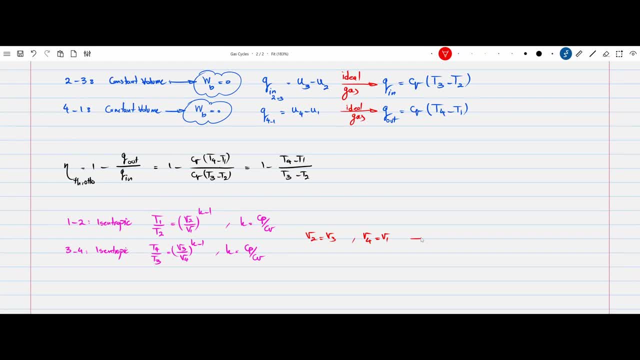 V4 is equal to V1.. This means V2 over V1 is equal to V3 over V4.. Now let's look at the next problem: V4 is equal to V3 over V4.. V4 is equal to V3 over V4.. 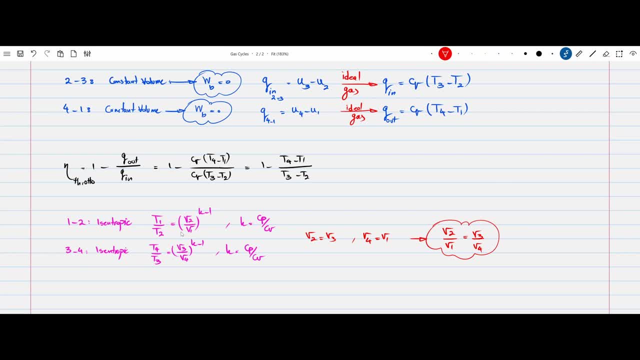 Now let's look at the next problem. V4 is equal to V7 over V8.. Now, taking this into account and looking at the pink equations, one can easily see that T1 over T2 is equal to T4 minus T3.. 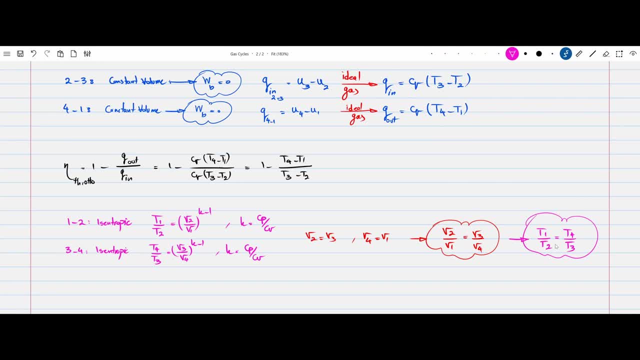 Okay, so this is very neat, but why do we need this? The reason is I can use this pink equation to simplify the efficiency equation for the autocycle. Look at this: If I play with this equation a little bit, if I factor out a T1 from the numerator and a T2 from the denominator, 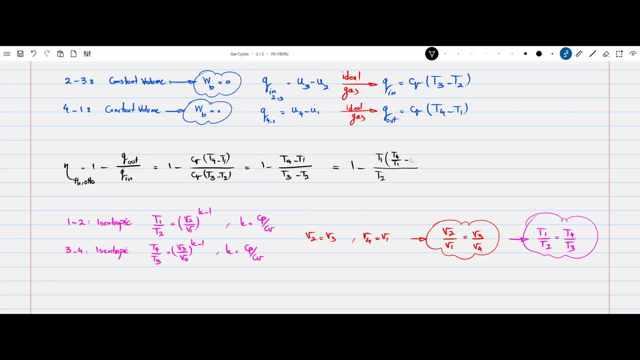 I get T4 over T1, minus 1 in the numerator and I get T3 over T2.. minus 1 in the denominator. Now if you look at the pink equation, you will realize that the expression in the parentheses in the equation on top 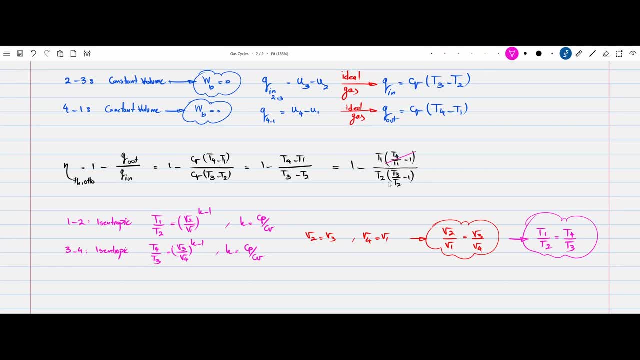 they are the same And so they cancel and you get 1 minus T1 over T2.. This is a very, very good equation, but we can improve it even further, Remembering that T1 over T2 is V2 over V1, raised to K minus 1,. 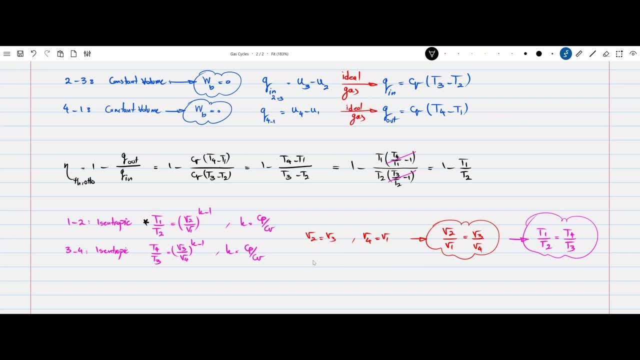 and remembering that V1 is Vmax and V2 is Vmin, you can check the graph a few times. You will see that V1 is Vmax and V2 is Vmin. One can say this is actually 1 minus Vmin over Vmax raised to K minus 1.. 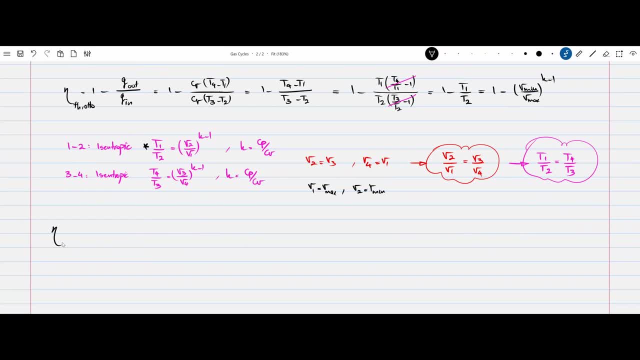 Now let's continue with this down here. So I have. the thermal efficiency of the autocycle is 1 minus Vmin over Vmax raised to K-1.. Remembering that the compression ratio is defined as Vmax over Vmin, 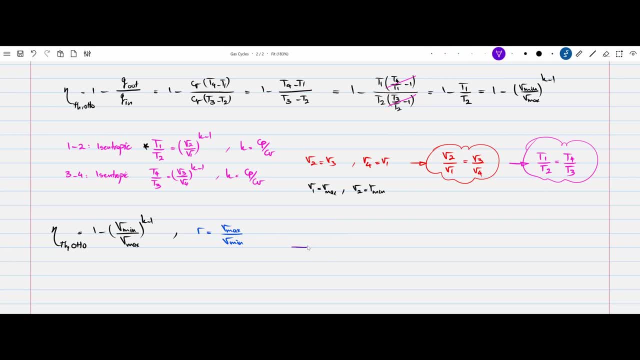 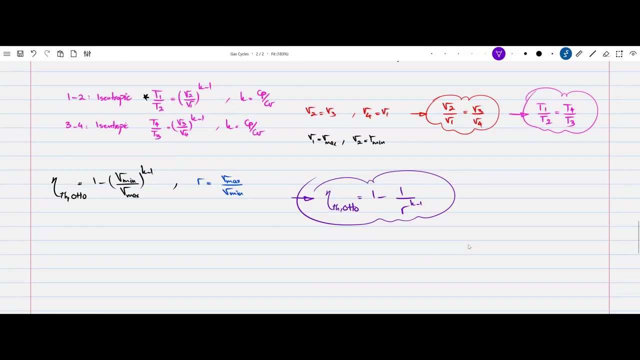 and combining everything together we get the thermal efficiency for the autocycle is 1 minus 1 over compression ratio ratio raised to k minus 1.. As you can see, the efficiency of otocycle is dependent on the compression factor R and the specific heat ratio Cp over Cv. If we draw the efficiency for a 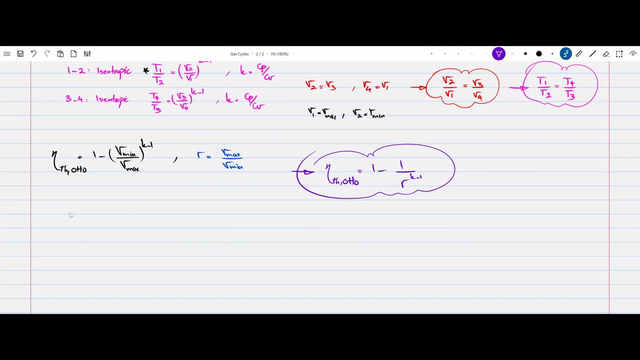 constant k as a function of R, we get a graph that looks similar to this. So this is the efficiency and this is R. You can see that by increasing R you get a very steep increase in efficiency, but after a while the increase in efficiency kind of dies out. Now, typically. 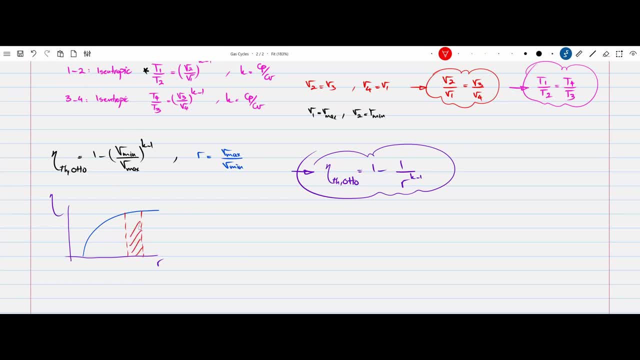 the modern age engines are designed with an R in the range of 8 to about 11.. So, by the way, if you look at the graph, you can see that the efficiency of otocycle is dependent on the compression factor R. By looking at this equation and this graph, one would wonder why not. 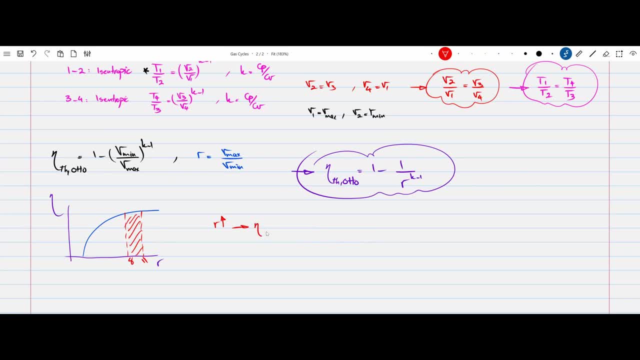 increase R as much as we can, because when we increase R, the efficiency also increases. This is true if you look at this equation and this graph only. But in practice, increasing R means that the pressure inside the mixture also increases. Now gasoline and air mixture is prone to self. 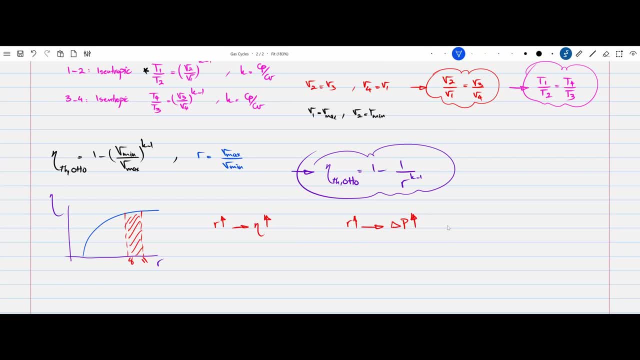 ignite at high temperatures and pressures, meaning that even before the spark actually ignites the mixture, the combustion starts to happen out of sync. This is a phenomenon that is sometimes referred to as an engine knock. You might have heard of it. An engine knock is when a premature 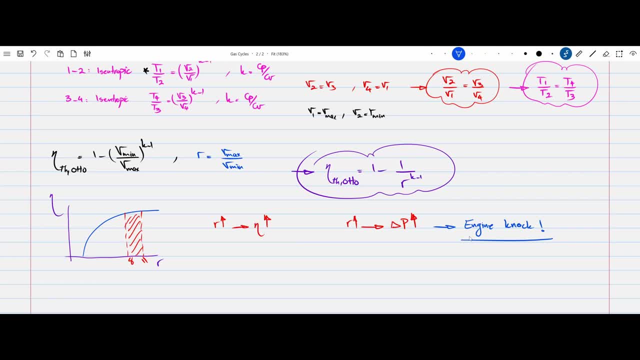 combustion happens within the cylinder Because it is out of sync with the rest of the components in the engine, specifically the crankshaft. it causes tear and wear on the crankshaft and it wears down the engine quite rapidly. So engine knock is something that we want to avoid. In order to avoid it, we have to keep R. 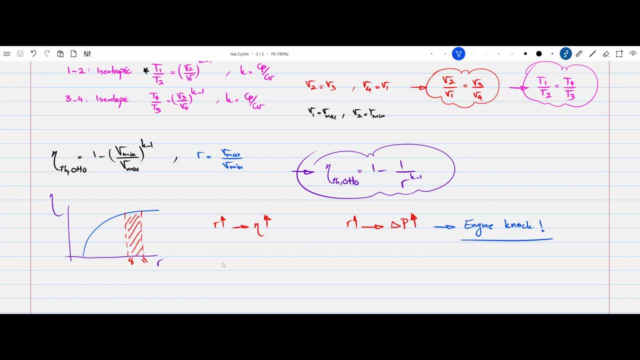 the compression ratio at a reasonable range. That reasonable range for the modern fuel that we have access to is approximately the same as the compression ratio. So engine knock is something that we want to avoid. In order to avoid it, we have to keep R the compression ratio, at a reasonable. 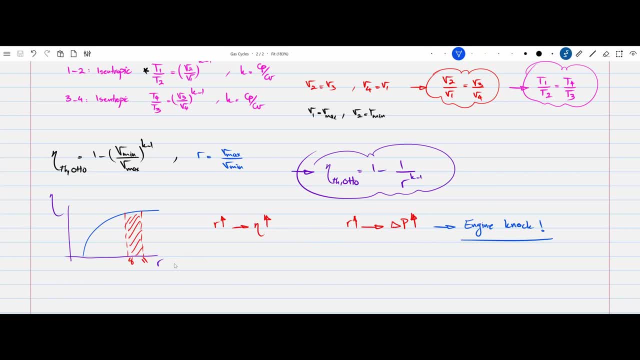 range. So engine knock is something that we want to avoid. In order to avoid it, we have to keep R, the compression ratio, at a reasonable range. So engine knock is something that we want to avoid. This is something with a carrying metal Tank and excited engine with easy acceleration. 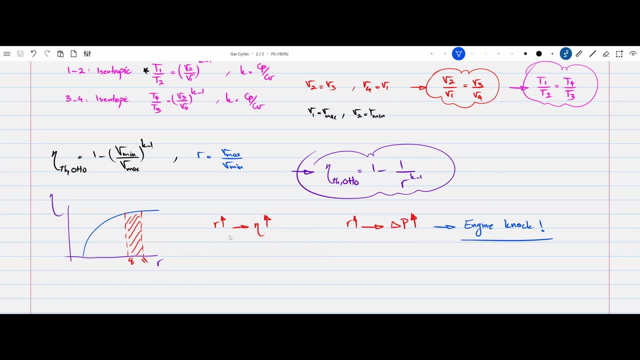 on both front without force. coyotes to areme shaped all-cylinder engines, very often spare parts, pumps and benches- All the components in this family are going to engine knock at lots of the sides already produced. benefiting from the car. they came with very small natural gas. 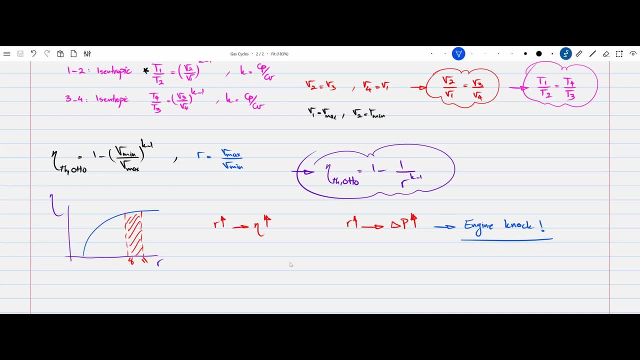 issues. So let's check the other two. all you need to know is remembering that the working fluid is an ideal gas, and also be very comfortable with how the processes are. Two of them are isotropic, two of them are constant volume. 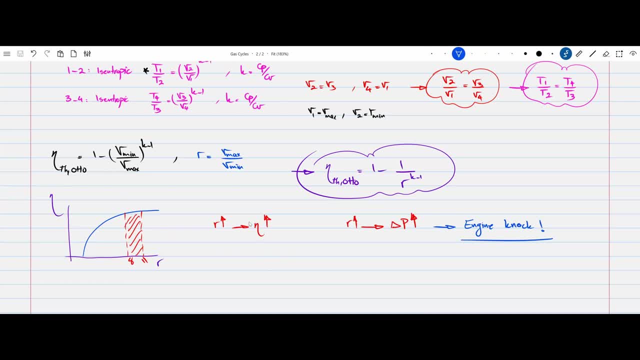 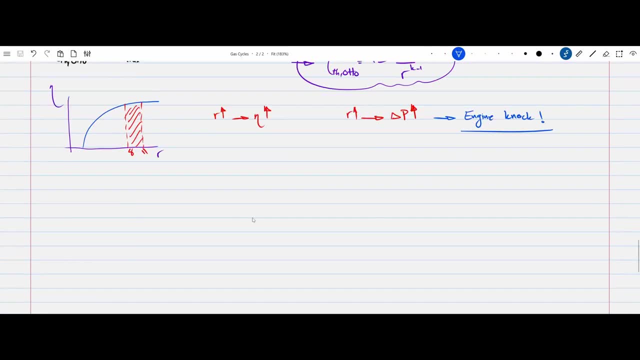 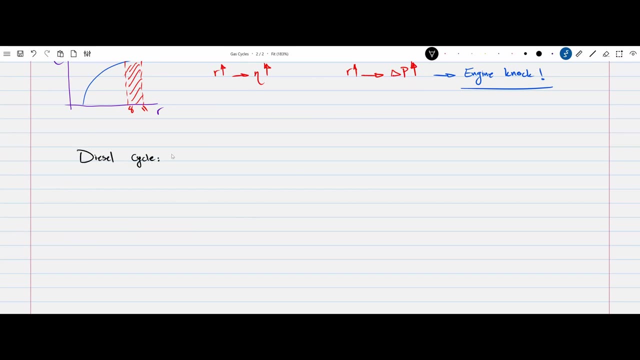 That is all you need to know to tackle problems from this topic. Now, before we end the video, there is one more cycle that we want to cover, and that is the diesel cycle, So let's start with that Now. the good thing is that we don't need to go through the details of every stroke again. 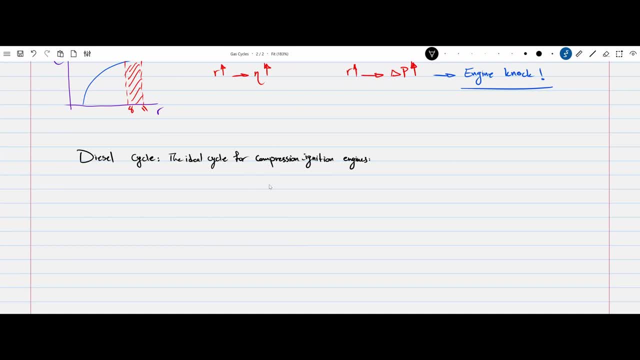 because it is pretty similar to the auto cycle. There is a little bit of difference, in a sense that we do not compress the mixture of air and fuel in the first stroke. In the first stroke we don't compress the mixture of air and fuel. In the first and second strokes we only compress pure air. The reason is, unlike the auto cycle, we are not relying on a spark anymore. So there is no spark. We are relying on the ability of air and fuel mixture to start the ignition automatically at high temperatures and pressures. 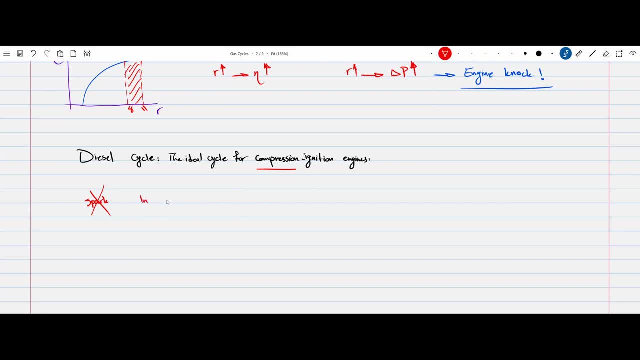 We are going to rely on that. Now. this compressed air is experiencing high pressure and high temperature. Now, at this moment, when the piston is at the TDC top dead center, we inject the fuel into this high P, high temperature air. 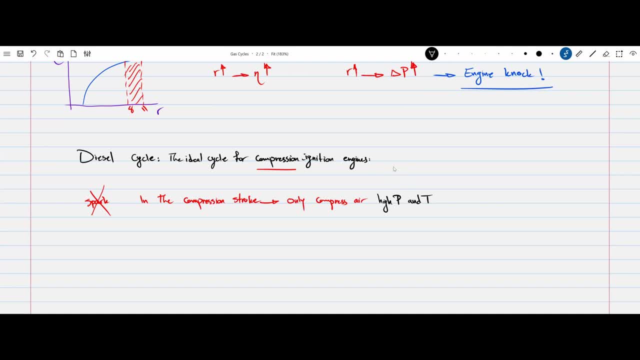 The moment you do that, because of the high pressure, the fuel starts to combust. Now, when this combusts, we are going to inject the fuel into this high P, high temperature air. Now, when this combustion happens, the piston has already started to move down. 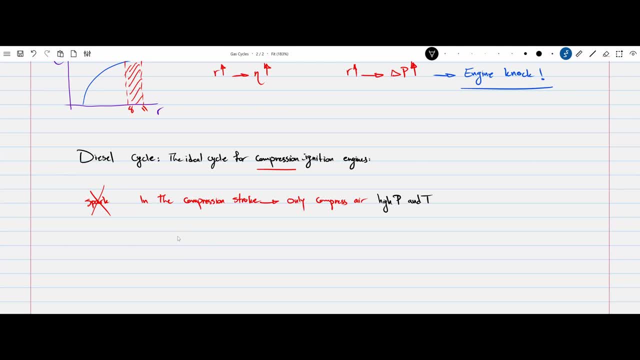 Remember, there is no spark and there is no instantaneous combustion. This is a continuous process. The piston has already started to move down when the process of burning starts. So that is the difference between the diesel and the auto cycle And you can easily show it on a PV diagram. 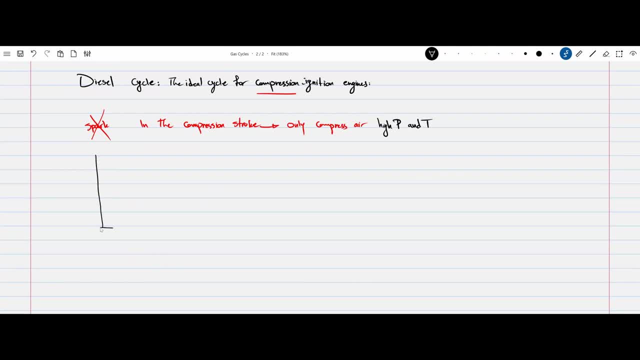 Let me show it to you. So again, let's say this is P and this is V, And we are looking at the cycle. The first stroke, the compression is kind of the same. You start from point one and you go to point two. 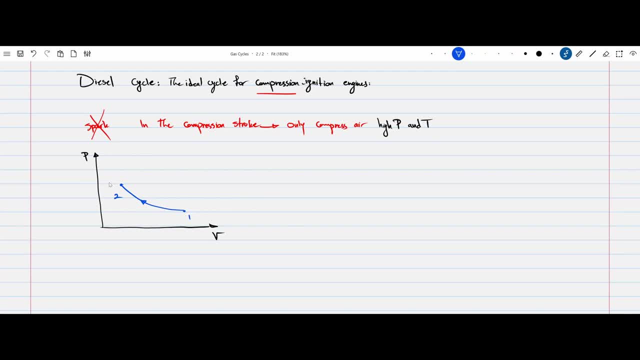 From the bottom dead center all the way to the top dead center. Then, when the pressure and temperature are high, you inject the fuel in. As I said, the piston has already. It has already started to move down while the combustion starts to happen. 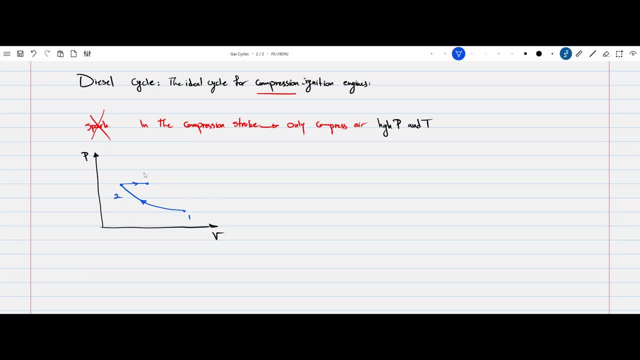 So for a brief moment, in the combustion process it is as if the process is constant pressure. When that is done, when the heat addition is done, the rest of the expansion happens, just like the auto cycle, an isentropic expansion, And we reach point four. 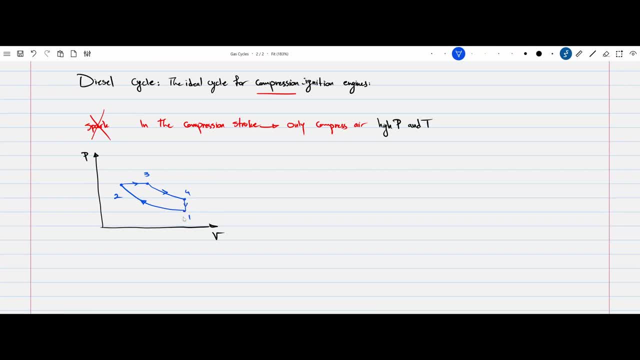 And after that is just a constant volume heat. This is called a projection or, as we know from practice, this is when the exhaust leaves the cylinder. So the only difference between an auto and a diesel cycle is that process. two to three, which is the heat addition process, is now constant pressure. 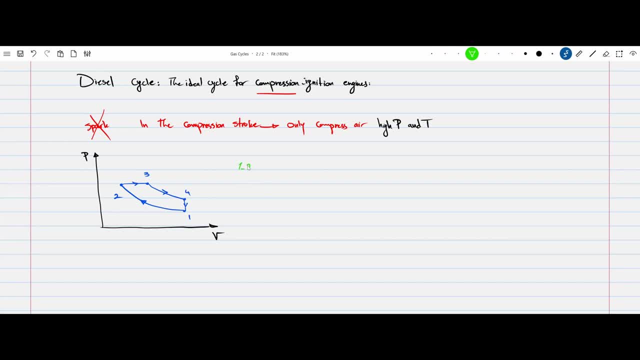 So let's write down the processes here on paper. So one to two is an isentropic compression, The sån that we draw out, which was contain a month and 10 days. In this particular example, we're looking at a single- ح primeroの斨伏0,. 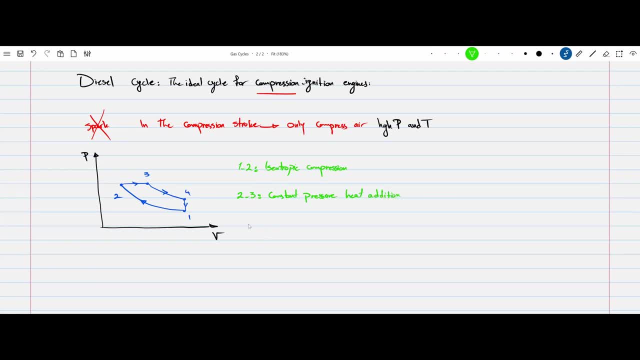 theization process. One service is a constant pressure heat addition. Then we have two additional kind of heat, But we've already seen these two stick together, which I've shown in previous videos. It's not just that I say four to one constant volume heat rejection. 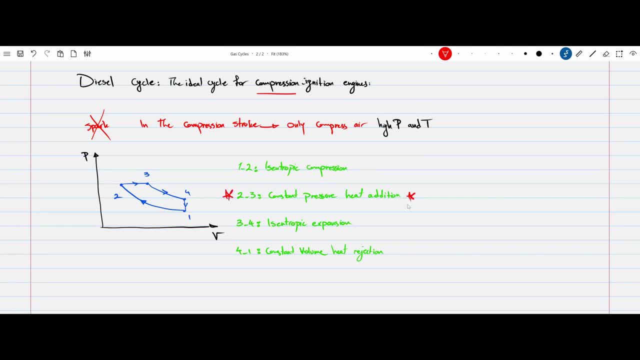 See, the only thing that is different is process two to three. This is where Q in happens and this is where Q out happens for our cycle. I'm going to show the TS diagram here as well, before we start dealing with the equations. So the TS diagram again. 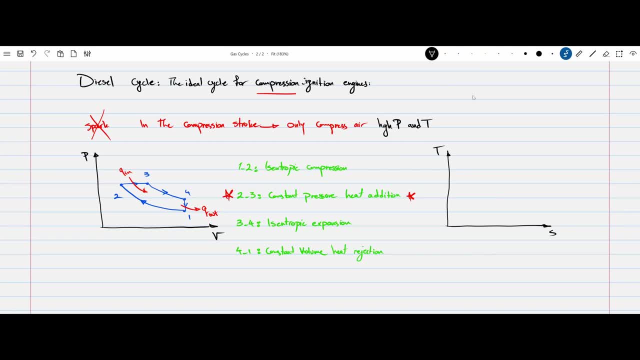 is very, very similar to the Otto cycle. We start from one to two, an isentropic process. So keep in mind S one is equal to S two. Then we have a constant pressure process From two to three. then we have a isentropic expansion. 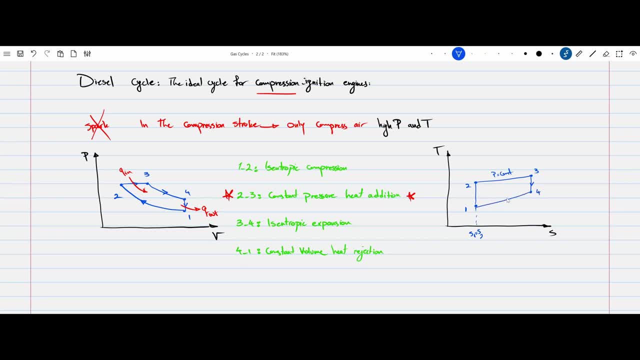 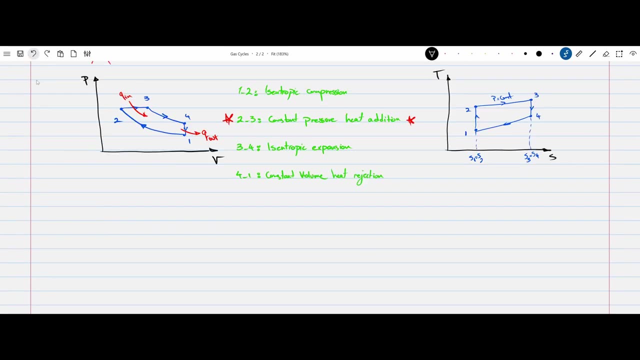 three to four, and then we have a constant volume heat rejection four to one. So keep in mind that S three is equal to S four, Putting the arrows so that we know where the cycle moves. Okay, so next thing that we want to do: 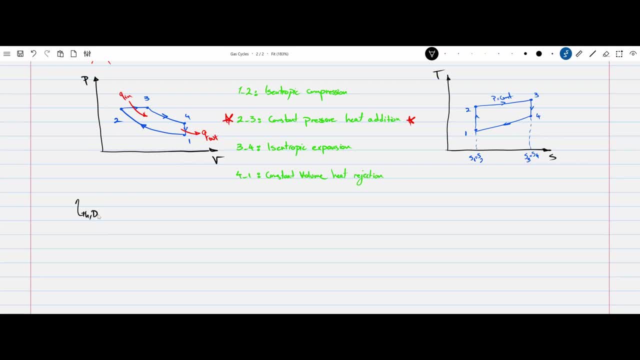 is coming up with an equation For the efficiency of a diesel engine. Again, we can define it as one minus Q out over Q, in The only difference. again, I want to emphasize this because it is important and is really the only difference. 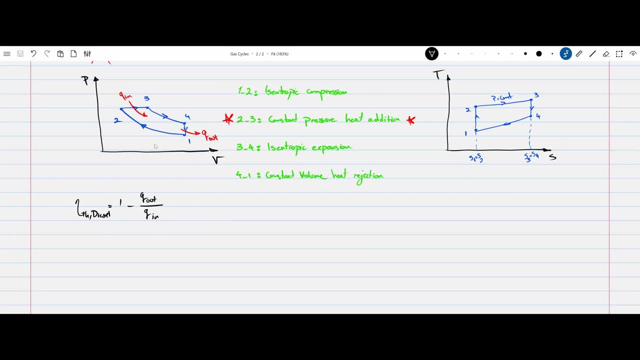 between diesel and Otto is that Q in now is a constant pressure. Again for every process. the first law of thermodynamics holds true. So that means for every process Q net minus W net is equal to the change of internal energy. 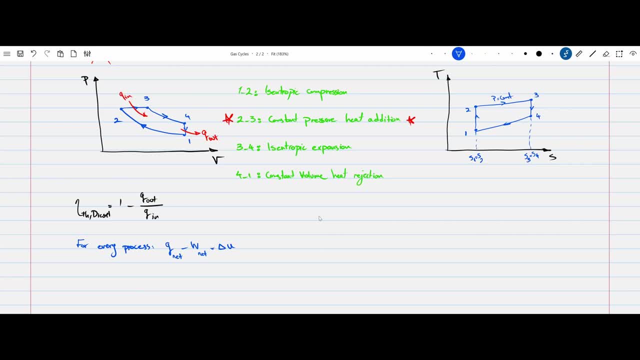 With that in mind, let's now talk about process two to three. So for process two to three, I know that hey Q is coming into the system, but this time this is a constant pressure process, So I have boundary work. 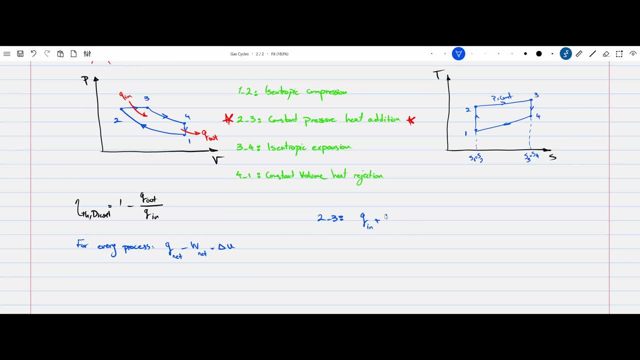 it's a constant pressure process. I know that the internalид does not come into my system And I can think of the pressure, which is the energy that's coming out of the system, which is F, which is the energy that's coming out of the system. 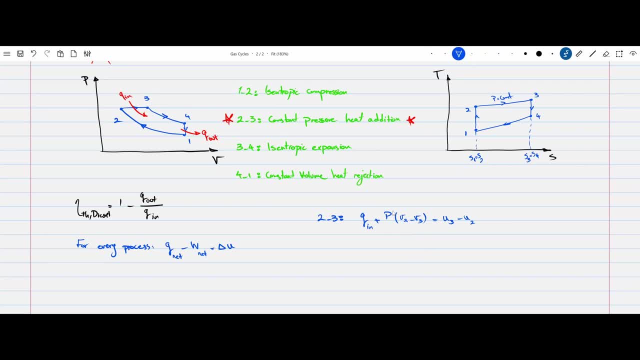 So I can do the process two to three and I can think of the temperature, which is one minus Q. So this is a constant pressure process. I will now talk about the airplane system. I'll just say one, two, three. 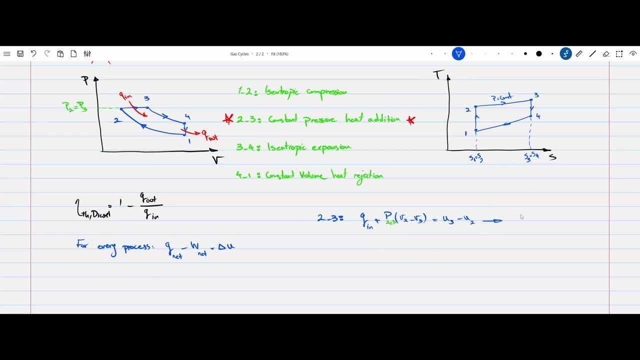 Okay, If you move things around in this equation, you get that Q in is U3 plus P3, V3 minus U2 plus P2, V2, right From before we know that this is the definition of enthalpy. so that is H3 and this is H2.. 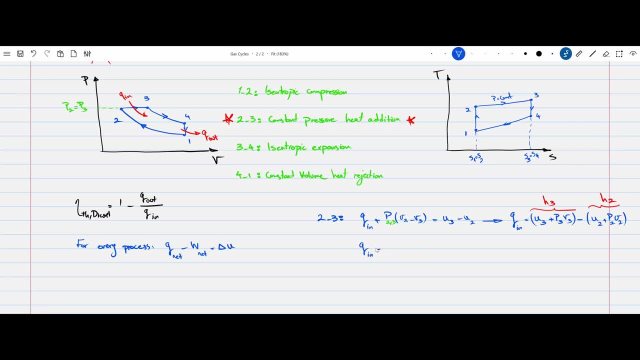 And so one can conclude that Q in for the diesel is H3 minus H2.. For an ideal gas, this is perfect For an ideal gas. we can approximate the temperature Change of enthalpy by CP T3 minus T2.. 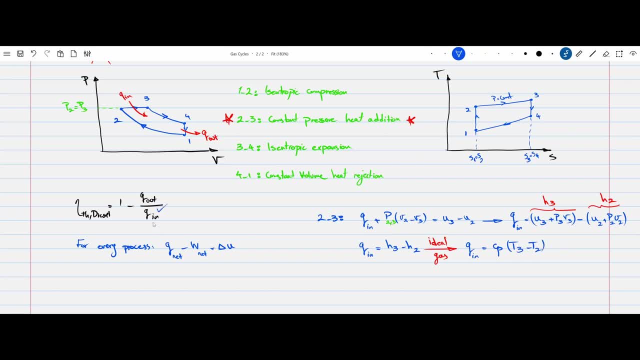 Very, very good. So I got Q in and Q out, the process 4 to 1.. It is exactly like the otocycle, which means Q out is this time CV. Please take note: This is now CV because it's Q. 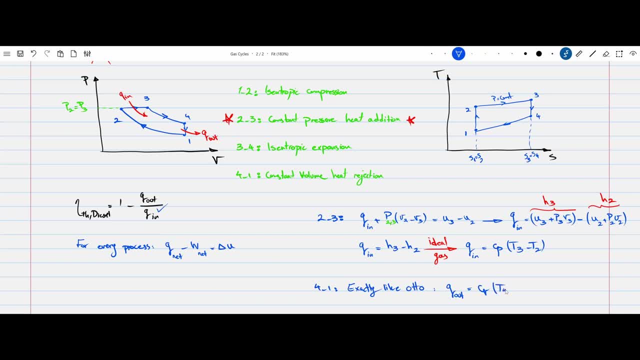 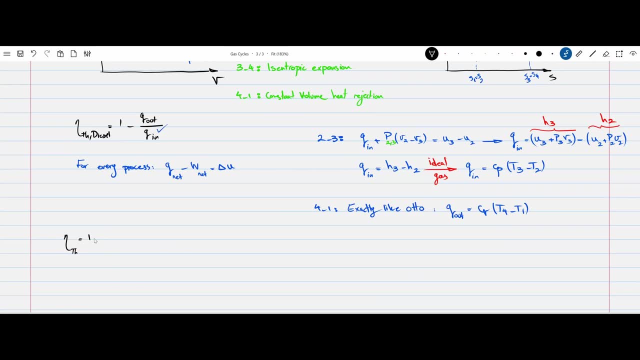 It's constant volume: CV T4 minus T1.. I can plug them back here. So the thermal efficiency for the diesel engine is 1 minus T4 minus T1 over CP T3 minus T2.. Now I'm not going to redo all of the calculations that we did for the otocycle, because you already know how to do it. 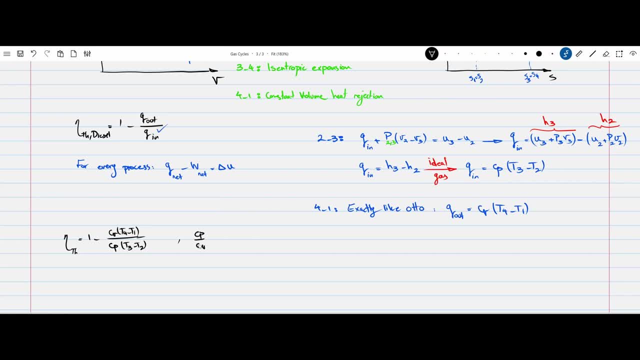 Keep in mind, Keep in mind that CP over CV, we show it with K, a specific heat ratio. Keep in mind that for the isentropic processes such as 1 to 2, T1 over T2, is V1 over V2, raised to K minus 1.. 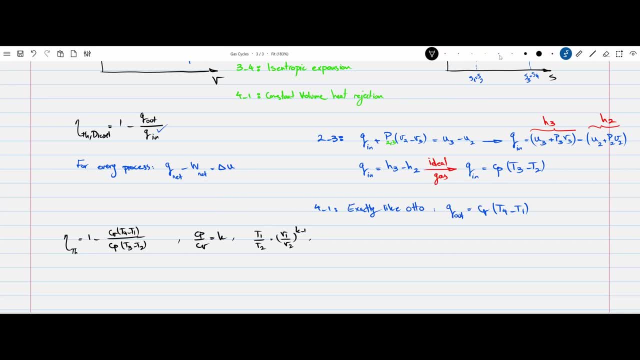 Keep in mind that that equation is true, And also introducing a new property calling the CO2.. The hot-off ratio: we show it with RC as V3 over V2, combining everything that you see here and more everything that we did in the otocycle, factoring out the temperature relating the 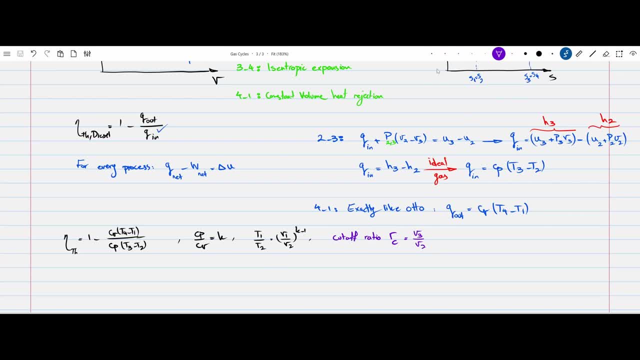 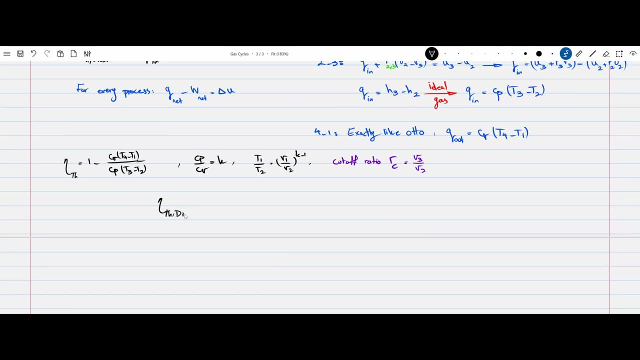 temperatures together through the isentropic relations one can finally get the equation for the thermal efficiency. So the thermal efficiency of the diesel engine, it is 1 minus 1 over R raised to K minus 1, so far, exactly like the otocycle times. this is where the difference comes in RC raised. 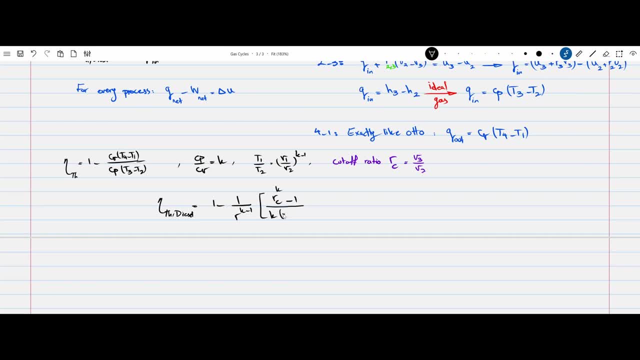 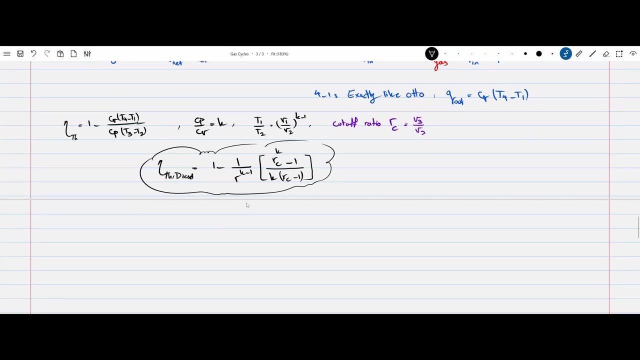 to K minus 1 over K RC minus 1.. Very interesting equation In the sense that it is very, very similar to the auto efficiency. However, it has an additional term. Let's take a look into that. I'm going to compare them here on this page. 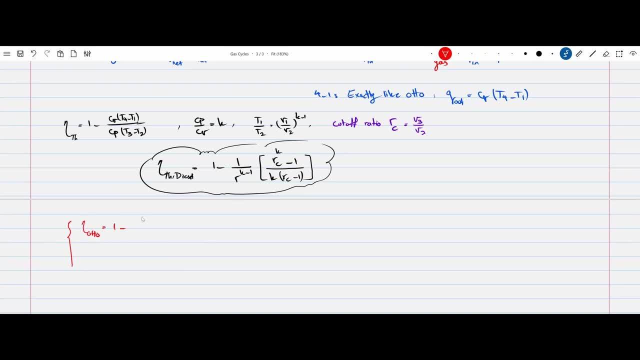 So for auto efficiency is 1 minus R over R raised to K minus 1.. For diesel it is 1 minus 1 over R. Obviously, if you want, you can add probability Rest to minimal function, including the SEC in the parole. 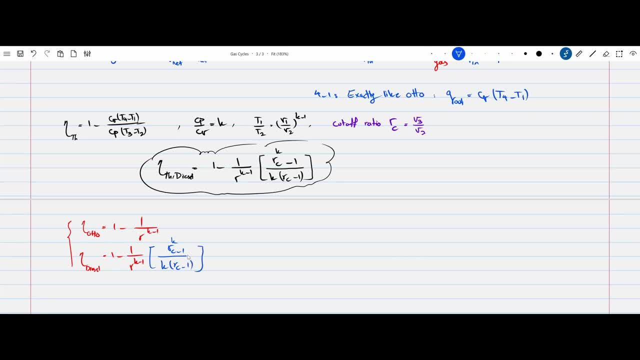 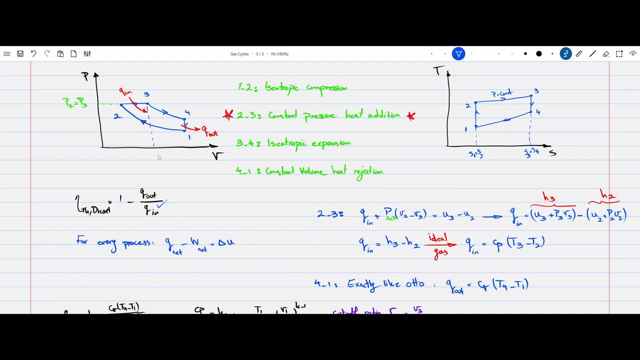 But here any kind of education exists. you don't know the mass, you just have to calculate the inhom모 both times and webecause this something. Now, this additional expression Is very interesting in the sense that if you pay attention to how we define cutoff ratio, 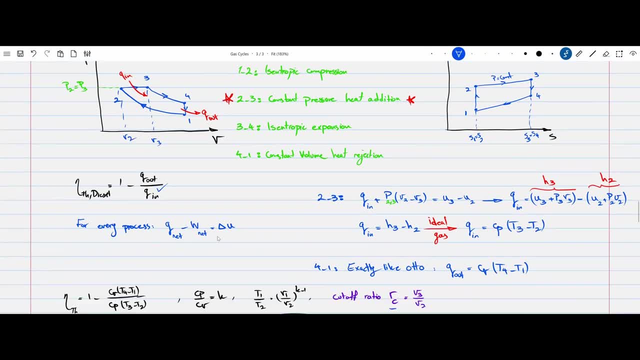 and if you take a look at the PV diagram, you see that V 3,. So if we take a look atそんな에, that is, mister, V3 is always greater than V2.. meaning that rc is always greater than 1..